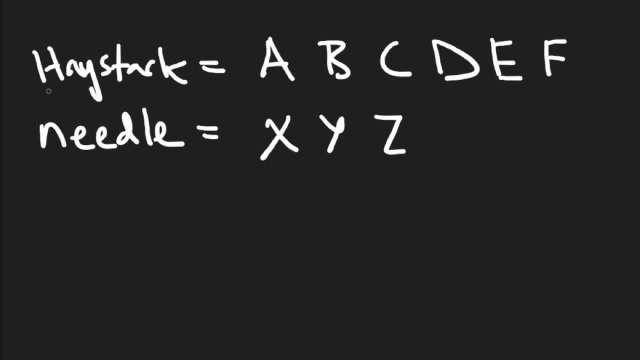 implement it. First, let's just quickly review through the brute force solution and kind of understand the motivation for this KMP algorithm. Remember, the brute force is going to take a substring. In this case we're going to call that the needle and the original entire string. 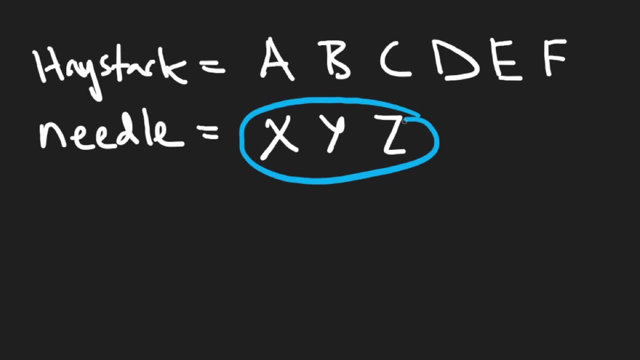 which we're calling the haystack for the context of this problem. We want to find a matching needle substring within the haystack right. First we check the first three characters. Do they match with the needle Nope? Then we check the next three characters. Do they match Nope? The next: 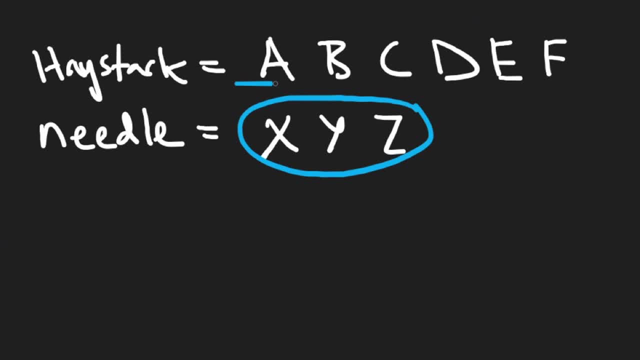 three, the next three, et cetera, et cetera. right, We're basically checking the first three characters, We're basically checking every substring of length three in the entire string. So that's what makes the time complexity really inefficient, basically multiplying both strings. 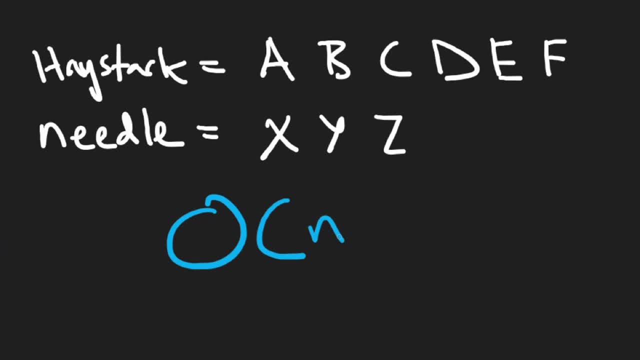 together. But in reality this brute force solution actually runs better than this. Take, for example, the two strings we have up above. First, we're just going to compare the first characters of each string right, A and X, to check if this substring is equal to the needle. 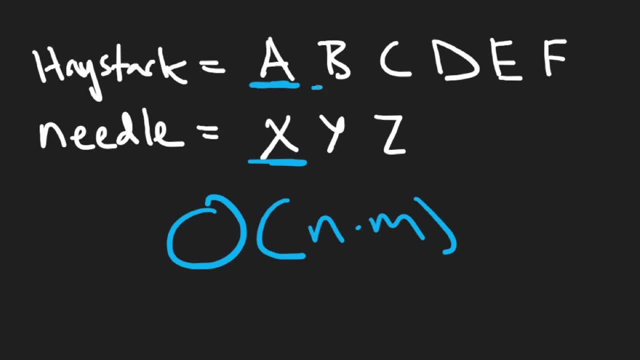 In this case, the first characters don't even match, So of course we don't even have to check the next two characters, right? So now we're going to check the first two characters, So we're going to check the next. We want to know if this matches the next three characters, So we just 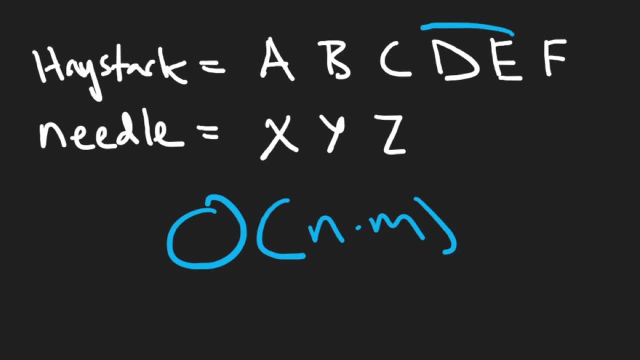 check the first characters, They still don't match. So we'll do the exact same thing with these three: The first character doesn't match. Then we check these three. The first character again doesn't match. So in this case this string was never found in the haystack And in reality, 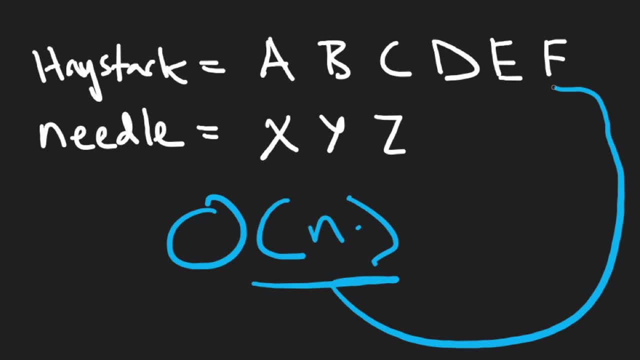 the time complexity was actually big O of N, where N is the size of the haystack. It wasn't very inefficient at all, which kind of shows you that KMP is not even super useful Most of the time. But let's take a look at an example where it will be very useful. So this is a very specific 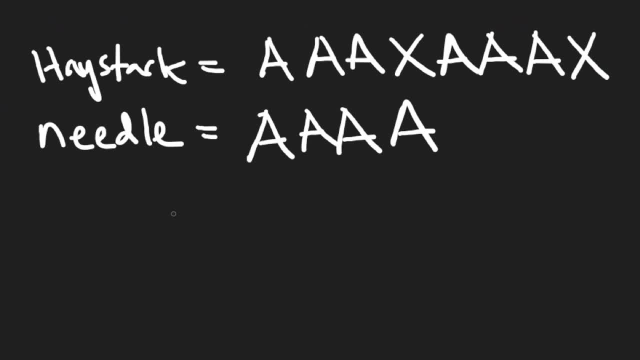 example, which kind of is necessary to illustrate the KMP algorithm? But in this case, if we try doing the brute force solution without KMP, we're going to check the first four characters. Do they match the substring we're looking for? Well, the first character does match The second character. 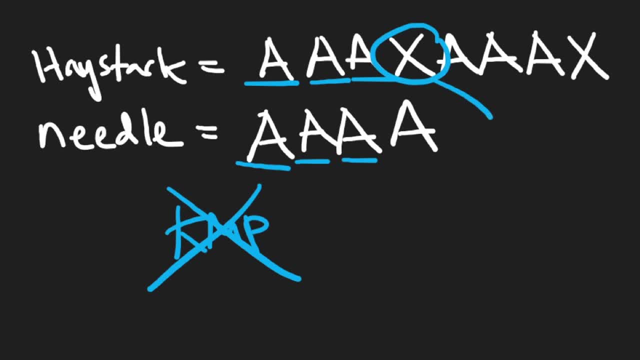 does match. The third matches as well, But the fourth is an X, when we actually want an A character. So this doesn't work. So we're going to go through the entire needle just to find out that the last character didn't match. That's pretty annoying. And next we're going to go through these four characters In. 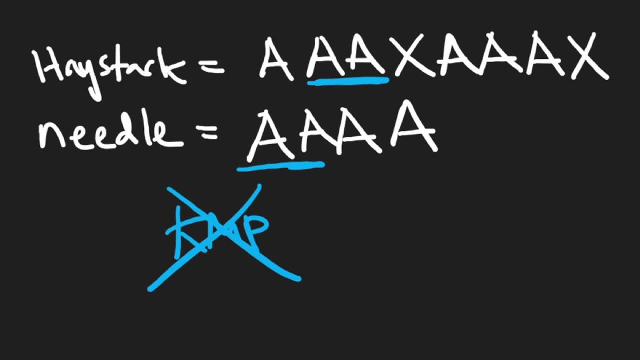 this case, we're going to check the first two characters, only to find that the third one does not match, And that's kind of the theme of these two strings, right. Next we're going to check here. OK, not too bad, We only had to check the first character which does match, But then the 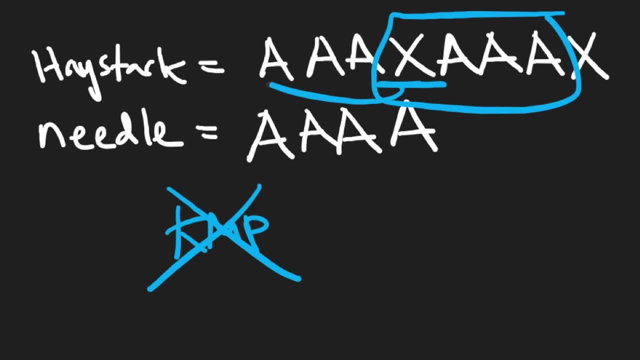 second one does not match. Next we check this: OK, the first one doesn't match, The X doesn't match. OK, not too bad. But then we kind of go through the entire needle just to find out that the third one matches. So we're going to go through all three characters just to check that. 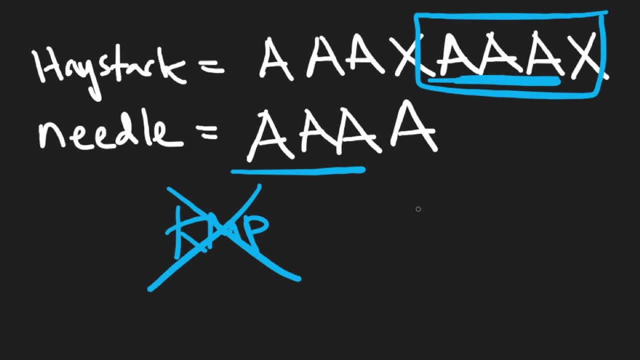 the fourth one doesn't match right. So this is an example where the time complexity- actually the runtime- is actually pretty bad. It's about N times M- And the KMP algorithm actually can solve that problem for us. It will ensure that the worst case runtime is going to be N plus M. 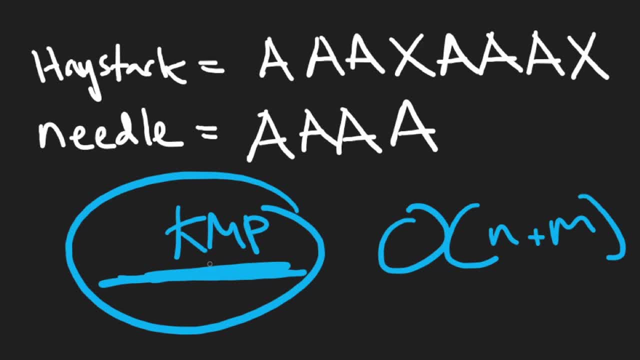 The downside is, it's very, very complicated, But I'll try to explain it in a way that you won't have to memorize it. So let's go ahead and try to explain it in a way that you won't have to memorize it, And then we're going to go through all three characters, just to check that. the fourth: 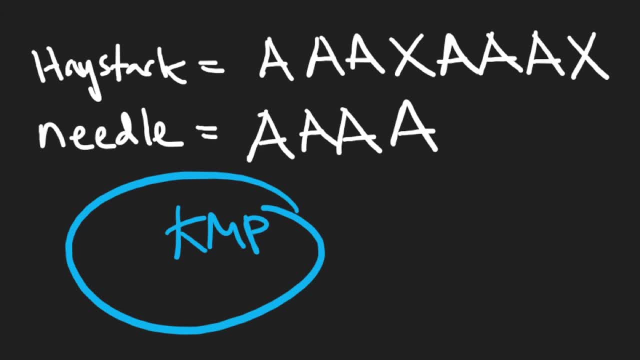 one matches. So let's go ahead and try to explain it in a way that you won't have to memorize too many of the details. You'll be able to allow your intuition to guide you to the solution. So the main idea is to cut out some repeated work by doing some pre-processing. So we saw that we 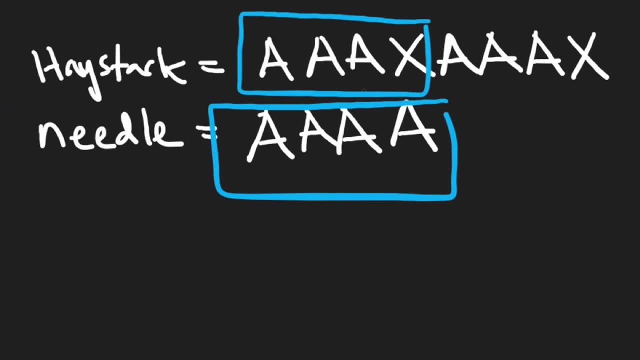 first compared the first four characters of each of them. The first three characters did match, but then we got to the fourth character which did not match right, And then we had to start all over again. Then we had to compare these with our needle And we had to start all over again. 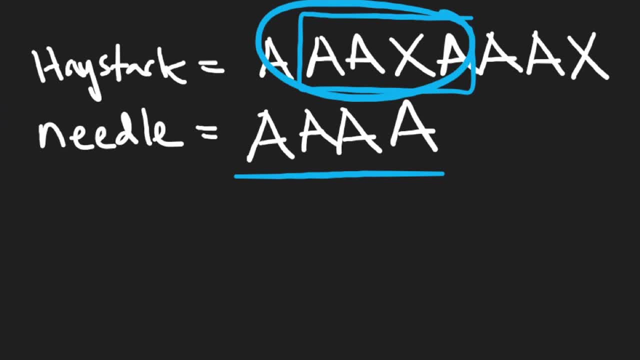 We had to start at the first character of this substring right. We had to go back to the beginning of our needle and here: But is that really necessary? Because, remember, it was this character that actually gave us trouble, It was the X character. These characters were perfectly. 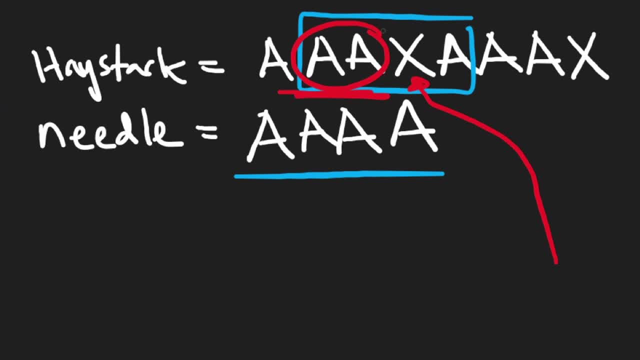 fine. And not only were these characters fine, these characters actually still match the beginning of our needle. This prefix matches this prefix, So why should we have to go through these characters again? In reality, our pointer in the haystack should still be at the X character, where we left off, where we found the mismatch. 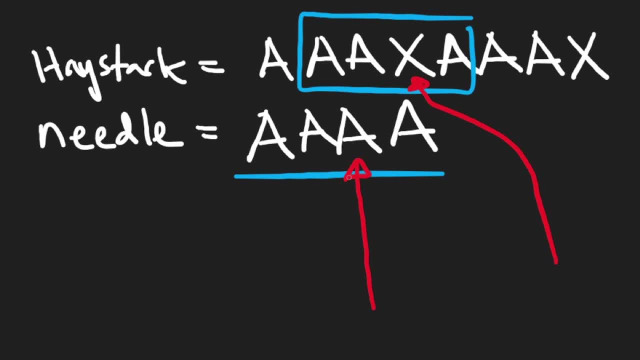 And our pointer in the needle should be over here, because the first two already match this. Can we somehow intelligently not have to do this repeated work again? And yes, there's a way. That's what the KMP algorithm is all about, And the first portion of this KMP algorithm is actually: 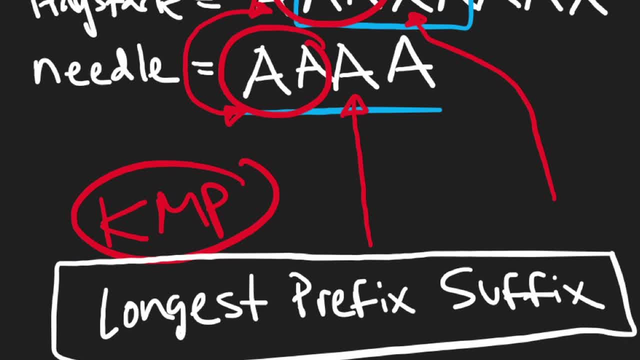 the it's called the longest prefix suffix portion. Let's just call it LPS for now, but it has to do with prefixes and suffixes. Basically, for certain substrings we're going to take a look at the longest prefix of that string. That is also a suffix of that substring. 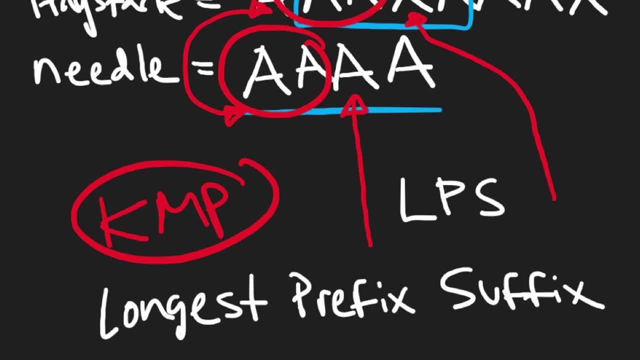 And you'll see why that's going to be really helpful. Basically, that's what's going to allow us to somehow intelligently take this prefix and already know that we don't have to read through this again, because it already matched a portion of the. 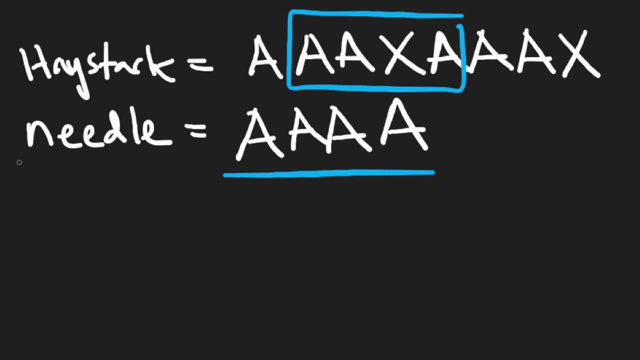 haystack and we don't have to go through it again. So for the needle itself, right, The pattern that we're trying to find within the larger string. that's what we're going to create the LPS array, for It's an array that's going to be the exact same size as the needle. What each index of this? 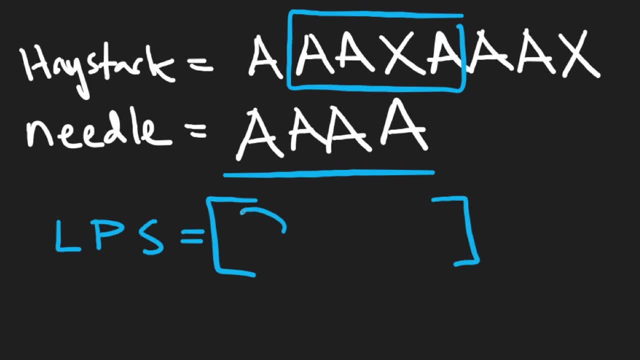 is going to represent is it's going to correspond. So, for example, the first position of the LPS is going to correspond to this substring, The second index of LPS is going to correspond to this substring, The third is going to correspond to this and the fourth is going to correspond to. 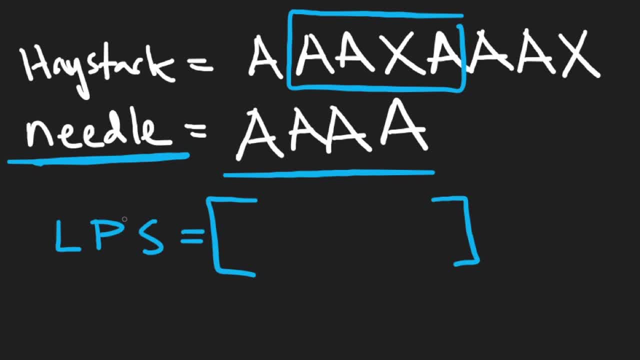 this, So basically every single prefix of the needle. So this is our substring portion And for the substring, we want to know something about it. We want to know the length of the longest prefix of this little substring over here That also happens to be a suffix, By the way. 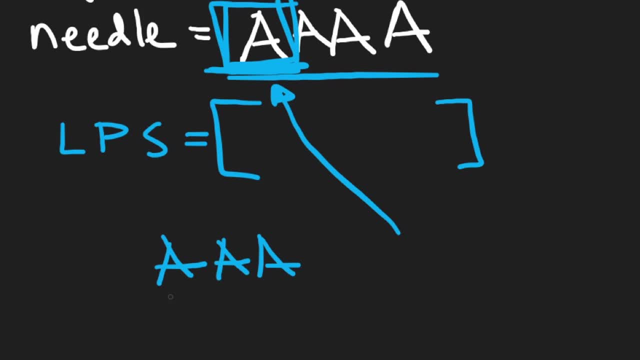 let's just say this is our string. A prefix is every substring starting at the beginning. So this is a prefix, right? Just the first character, The first two characters is a prefix. The first three characters is also a prefix And, by the way, a suffix is basically the opposite: Every. 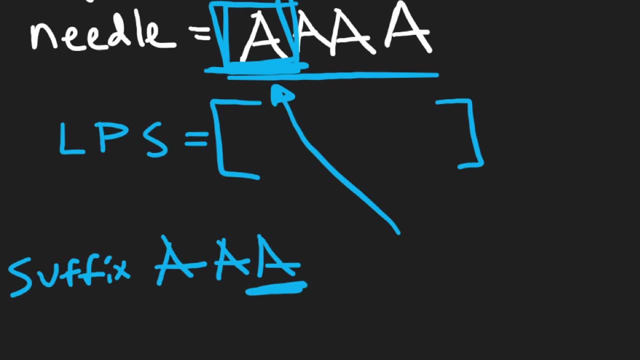 substring that ends at the last character. So this last a character is a suffix, The last two characters are a suffix and all three characters are a suffix. So we want to know the length of the suffix. We want to know, for this little substring with just a single a, what's the longest? 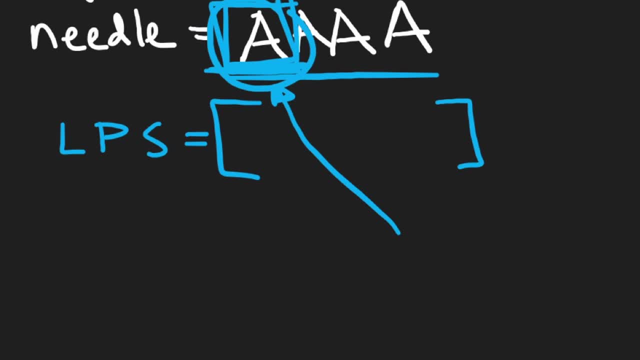 prefix. that's also a suffix. Well, the string itself, a, is a prefix and a suffix, right? So can we just take the length of that and say one for the first position? Well, not exactly, because I kind of lied. We're not just looking for the longest prefix. That's also a suffix. There's. 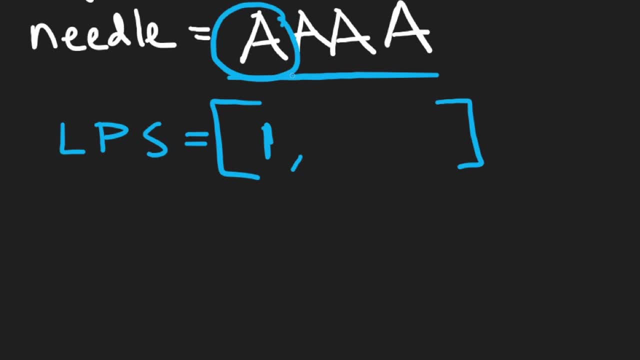 one catch, and the prefix itself cannot be the entire string itself. So in this case we can't put a one here, We have to put a zero, because the entire string itself can't be one of the prefixes and we only have a string of length one. So basically what we've. 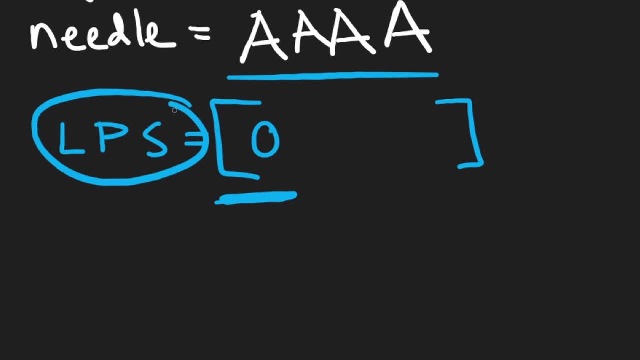 figured out is the first position of our LPS is always going to be zero. The next position is where things get a little bit interesting. So now the substring we're looking at is the first two characters, because this is the position that we're at. So what's the longest prefix of this? 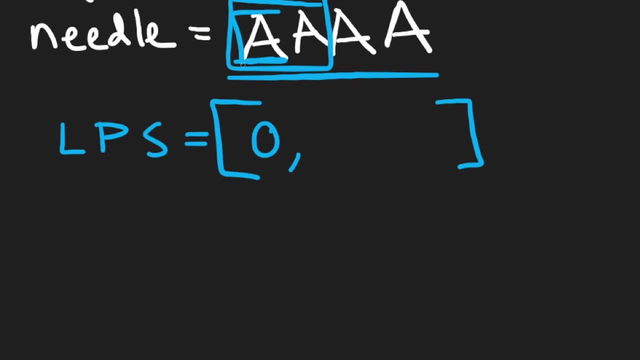 that's also a suffix. Well, the first character is the same as the last character, So we can say one and the next position. It's pretty simple in this example. So we're going to look at this substring, which is the first three characters, because we're at the third position of our LPS, So what's the longest? 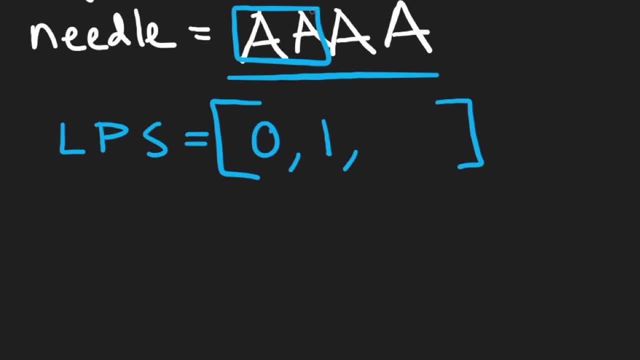 prefix. that's also a suffix. Well, the first two characters, right. The first two characters match the last two characters, So we can put a value here too. And then, when we're at the last position, we're looking at all four characters. The first three match the last three, So we can. 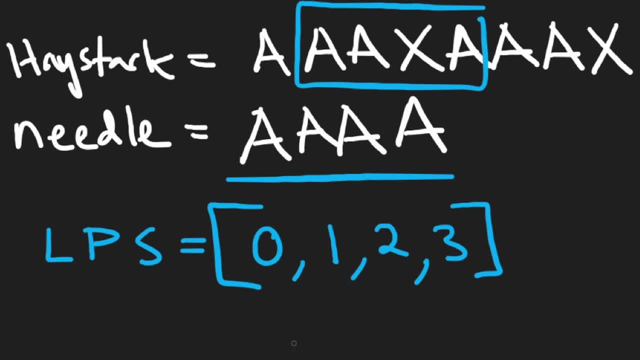 put a three in this position. Okay, we're not quite done with the algorithm yet, but we have kind of got an understanding of the first portion, which is the LPS longest prefix suffix portion. So what I'm going to do, for the first time in neat code history, is actually dual screen this. So now, 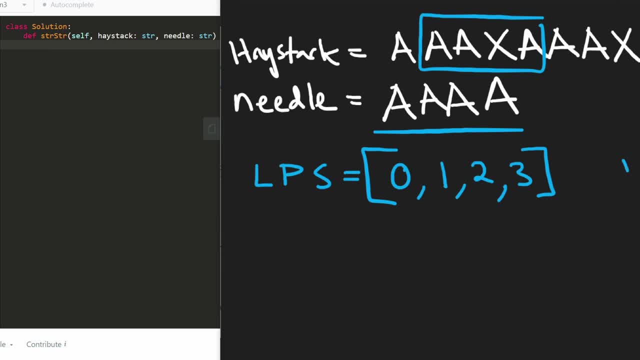 we're actually going to be doing the code at the same time as we look at the drawing, because this problem is so complicated. I think that's going to be really helpful for us. So first thing I'm going to do is just for the context of this leak code problem itself, if the needle happens to be, 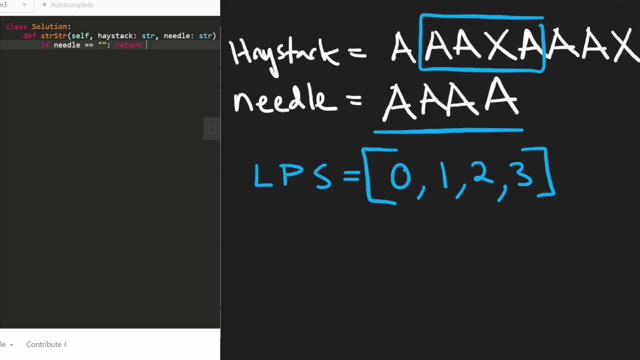 an empty string, then we have to return zero, saying that the first matching index we found was at index zero. But now we can get to the LPS portion. So we're going to create an LPS array. Initially, let's set it to all zeros and set it to be the same length as our needle array, right? 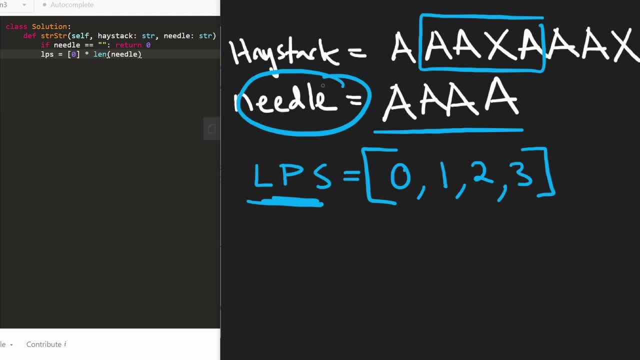 Because the LPS is always going to be the same length as the needle. Okay, so now we're actually going to use two pointers for this problem. We're going to use the previous LPS pointer, which is is basically going to tell us the length of the previous longest prefix sub suffix. quite a. 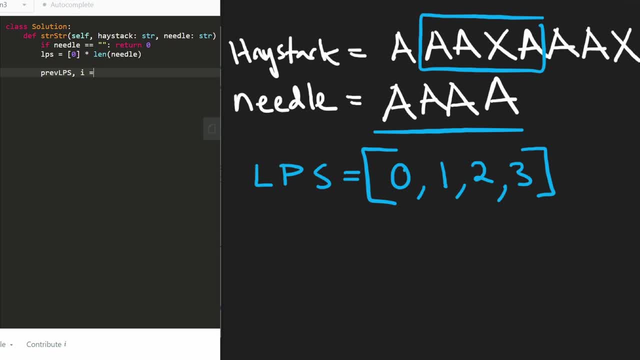 complicated term And when we're also going to have a second pointer, I, which is going to be the current character we're looking at. So originally, the previous LPS is going to be zero and I is going to be one. The reason we're saying that is because, remember, in this position, right? 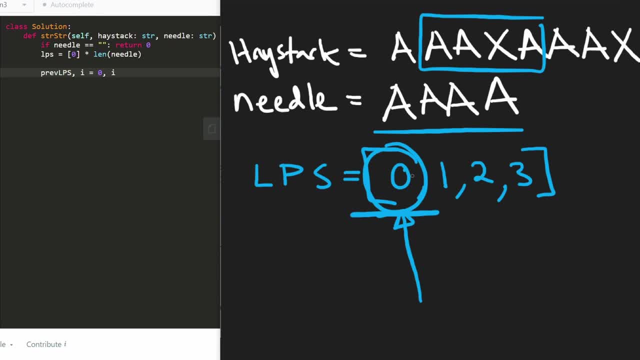 it's always going to be a zero right. That's why previous LPS is zero And our I pointer is actually going to be starting at one, At this index at least. even though this value is a one, the index of this is also a one. 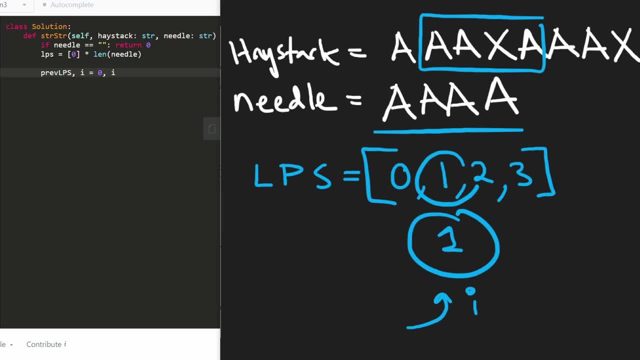 That's why our I pointer is set to this position. but we haven't figured this value out quite yet. So let's actually reset this thing to zeros. So now we can fill in the rest of this as we go And actually let's do an even more interesting example. So this is actually the example we're. 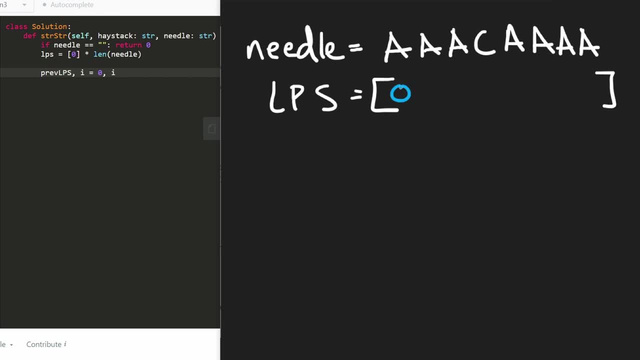 going to look at. We're introducing a C character because you're going to see why it's going to make this a lot more interesting and also a lot more interesting. So let's go ahead and do that more difficult. Don't say I didn't warn you. with this KMP algorithm It's quite complicated. So 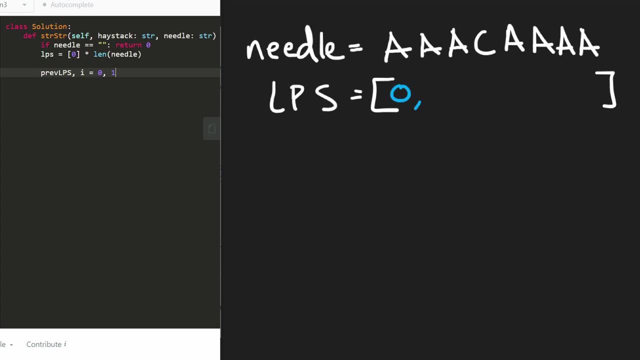 I set I equal to I, but we actually want it to be equal to one. So right, our previous LPS is going to be at zero and our I pointer is going to be at this index, looking at this character. So we're going to do a while loop, right, While I is less than the length of the needle. right, Because 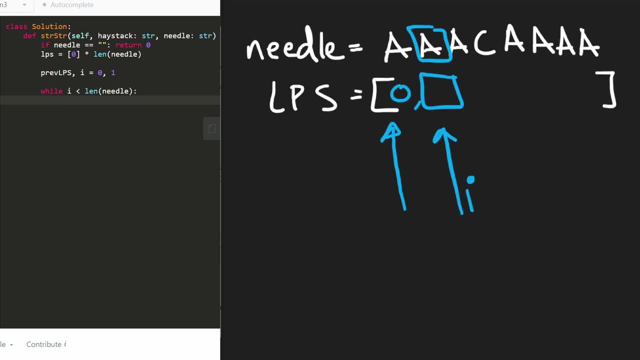 we're going through every character in the needle to fill in this LPS array, And so the simplest case is going to be if the characters match each other, So if the needle app index I is equal to the needle at index previous LPS. So what's going to happen in that case? Well, we're going to set LPS. 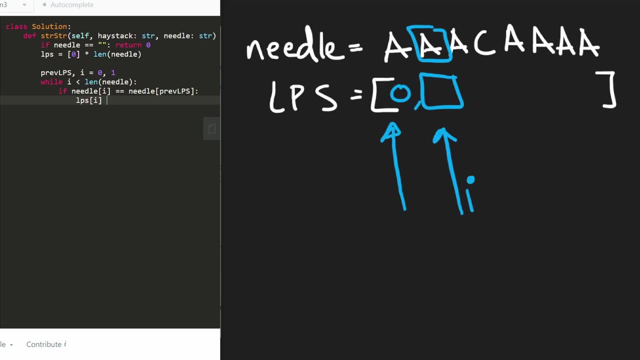 of I equal to the previous LPS plus one, And we're going to increment now the previous LPS by one, right, Because for the next iteration of the loop we want it to be incremented by one, because we just realized that these characters are. 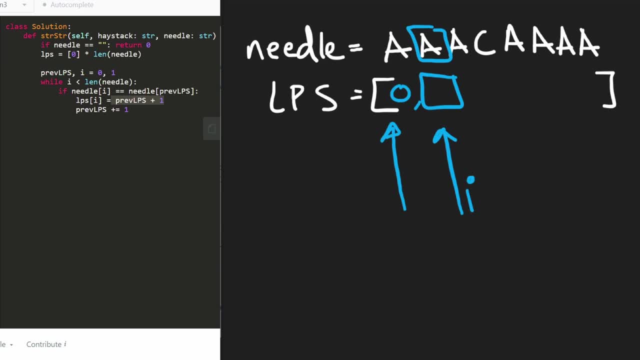 equal. So we set the current LPS to previous LPS plus one. So the value in here is basically what we're replacing the LPS with. And of course we want to take this I pointer now and look at the next character at the third index. So we're going to go ahead and say I plus equal to one. Now these 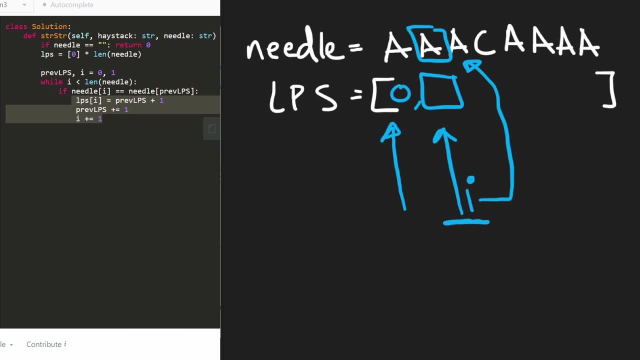 three lines of code actually are kind of complicated. Let's kind of go through this drawing and understand how to do that. So we're going to go ahead and say I plus equal to one, And of course we're going to reicki them To do that. we're going to how to plant them. So how is it? 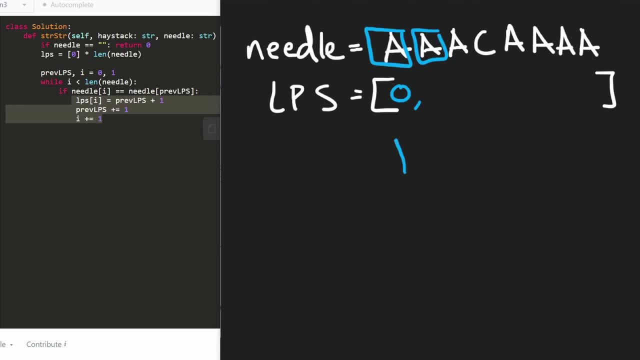 going to run first of all. well, we're going to compare these two characters. right. previous LPS is your eyes here. these two characters are equal. What does that tell us? Well, that tells us that this is the prefix, this is the suffix, since their equal, we're going to take this and set it. 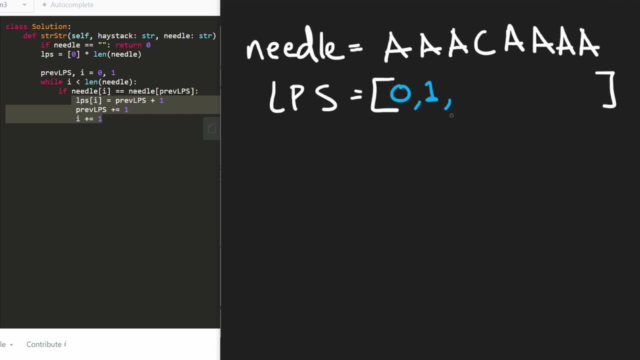 to be one. Now what's going to happen on the second iteration of the loop? we set previous LPS to be at this position And we set I to be at this position, right, We incremented both of them to be the prefix. 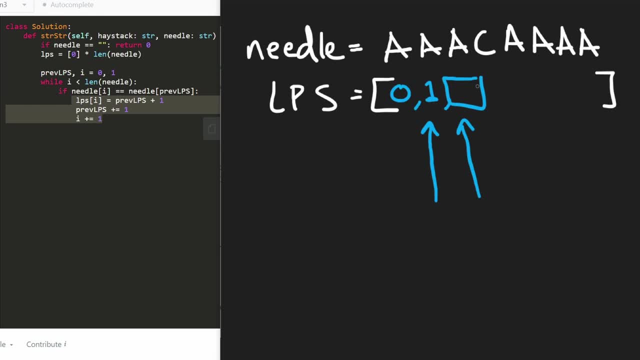 by one. Now we're looking for the LPS value in this spot. So, again, according to our algorithm right now, we're going to compare these two characters. They are equal again. So what are we going to put in this spot? We're going to take the previous LPS and add one to it, So we're going. 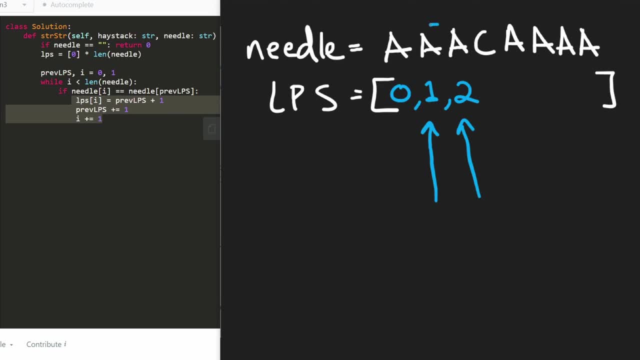 to end up putting two here. right, That makes sense. These two characters are equal to these two characters, So two is the right value to put here, because, remember, we can't use the entire string as a prefix. but how did this magically work? Why are we adding the previous LPS value? 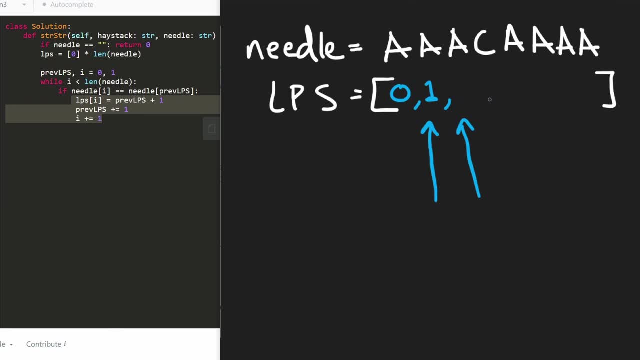 plus one. Well, that's the slightly difficult part. Let's explain it. First of all, when we determined that the LPS value here is equal to one, what we actually determined was that this character, this prefix, is equal to this suffix right, This character. 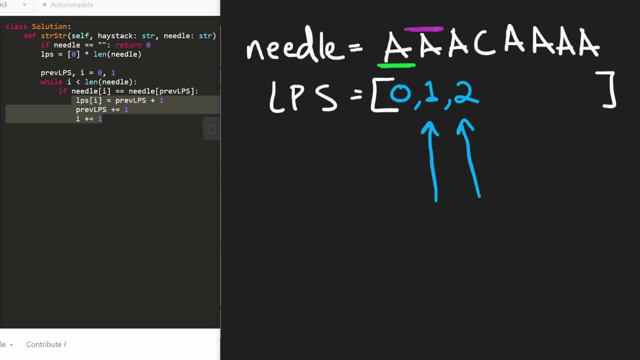 is equal to this character, this prefix, this suffix. so now, when we're in this position- right, we're not all- we're not manually going through the first character, uh, setting is checking if it's equal to this, etc. etc. right, we're not starting all the way at the beginning because remember our previous. 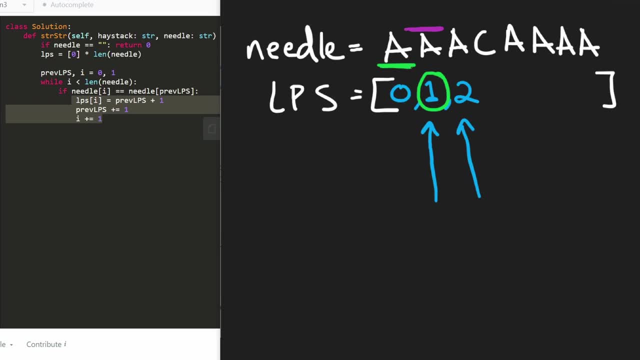 lps value is one that tells us that this character already matches this character. right? so we don't even have to check this one, because if we compare this value and it happens to be equal to this value, we already know that this matched that. so therefore, if this matches this, then we can just 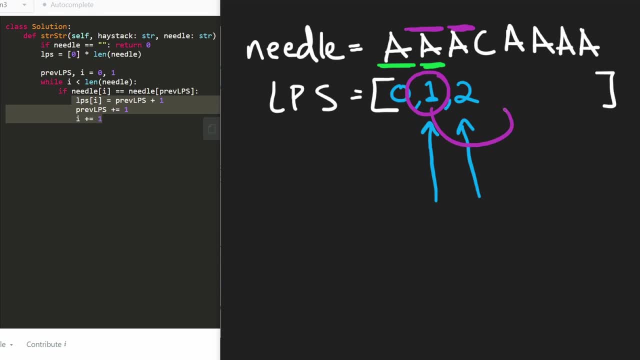 take the length of the previous lps and add one to it. right, and this seems really complicated. maybe you have an easier way you could implement this, but remember our goal is to keep the time complexity to be n plus m, so we have to be able to. 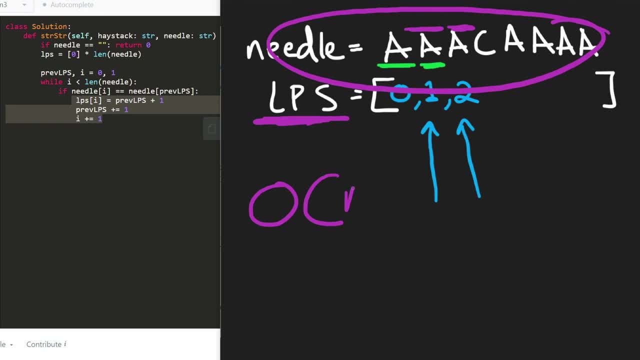 do this needle lps algorithm in uh o of n time where let's say, n is the length of this and actually i'm going to be referring m to be the length of the needle. so that's basically why we use the previous lps index or the previous lps value to tell us what index to compare it to. 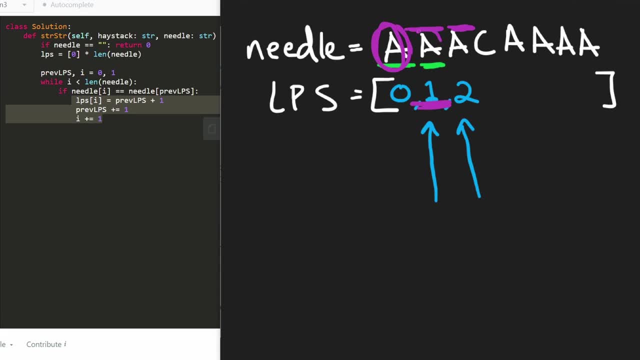 because if this is one, that already means that the first character matched this. so it's complicated. but let's quickly go through the rest of this example, because it's about to get a little bit more complicated, because now we are going to have our previous lps pointer be over here and our i pointer is: 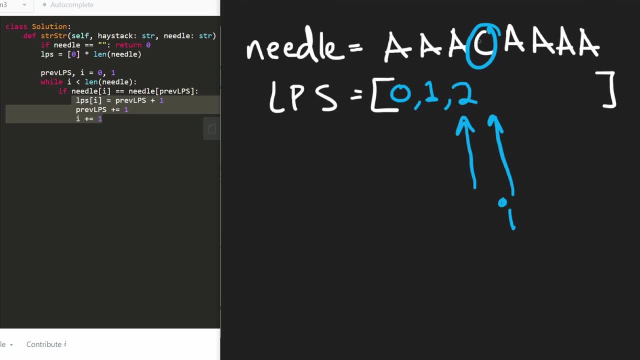 going to be over here and this is going to be the first time where we actually see that the two characters don't match each other. clearly we need to accommodate our code to deal with this right, because right now we only have the case where they do match each other, and within this else case we 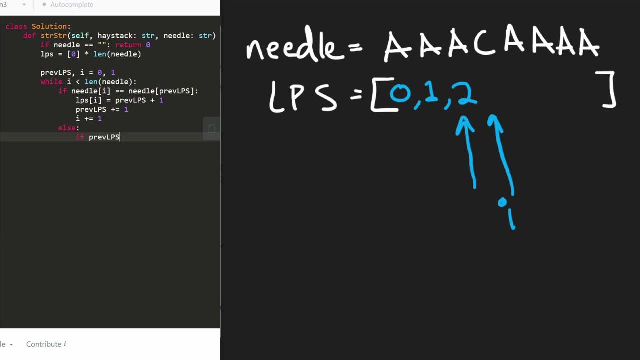 are going to have one more conditional and it's going to be if previous lps is equal to zero and the else condition where it's not equal to zero. because it's going to be a little bit different, because, as i was kind of talking about right this position, so we know that the previous 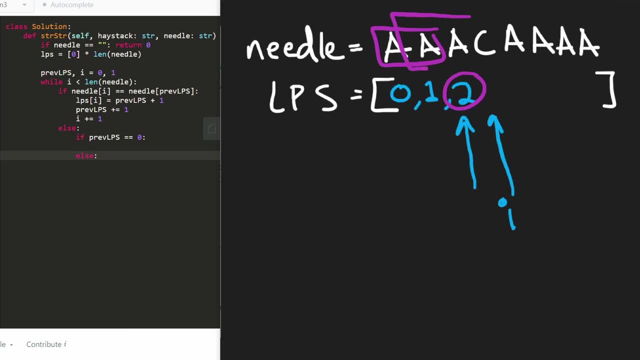 lps is two, that means we already know this matches these two characters. so we only have to compare these two and check if they're equal. if they are equal, we can take this value two and add one to it and set this to three. but what happens when they're not equal, which is the case right now? 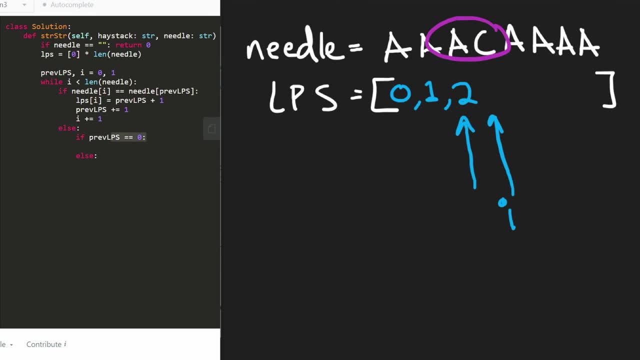 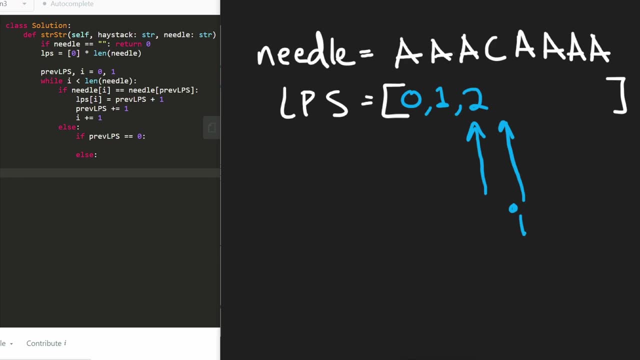 well, first of all, let's let's consider our first case: if previous lps was actually equal to zero, because right now our previous lps is equal to two. but let's consider a different example. let's just change this really, really quickly. so let's just consider a different. 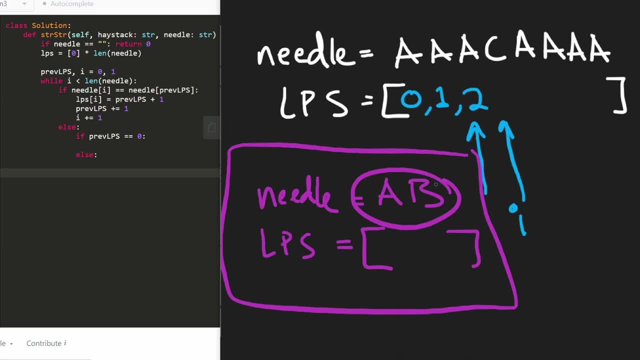 example, for a quick second, let's say we're doing the lps of this. we know that the first value is always going to be zero. so right now we're comparing this character with this character. are these characters equal? no, they are not. so we do our else case right and we look if previous 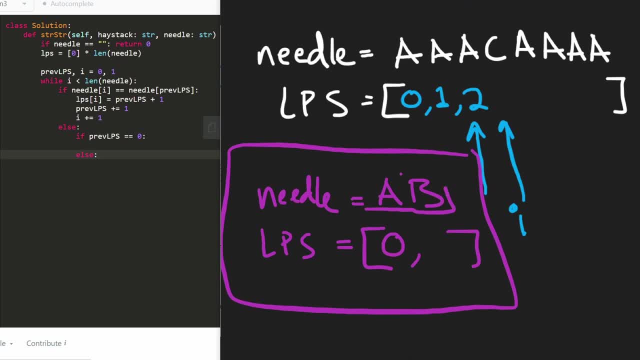 lps is equal to zero, meaning that there was never a prefix of this string. so we're going to have to look at the string that matched a suffix of the string. so that also tells us that the pointer that we're looking at is actually at the beginning, all the way at the beginning of the string. if even the 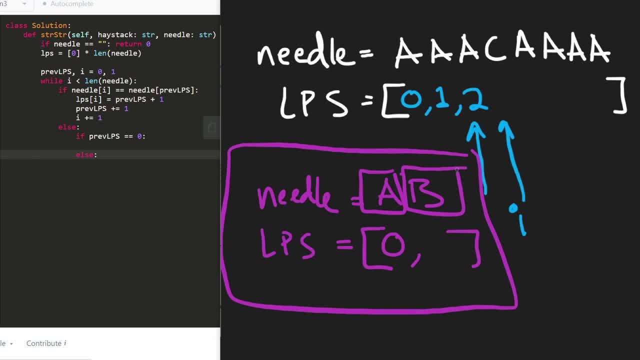 first character does not match the- you know last character, that means it can't possibly- we can't possibly- have a prefix that matches a suffix, right? so that means we can just put a zero here. so that's the simple case. we're going to say that if a previous lps is at zero, then we can set lps of i. 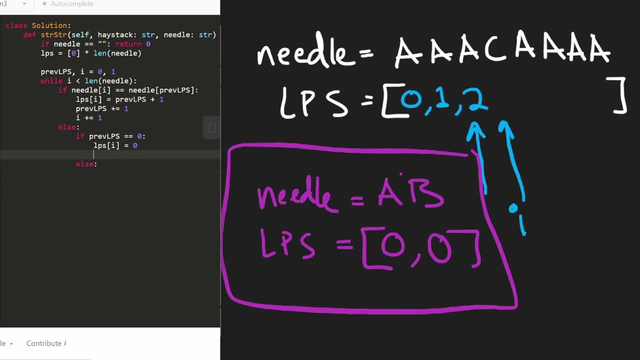 equal to zero. and also, let's not forget to increment our i pointer, because we don't want to get stuck in an infinite loop. so we have our previous lps here. that's what i'm going to use p to refer to. i is over here. the characters do not match each other, and previous lps is not equal to zero, right? our? 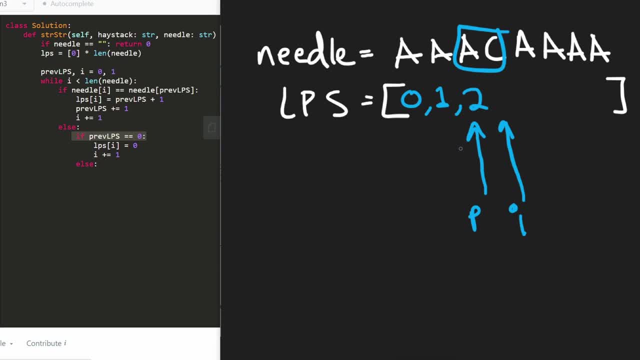 previous lps is equal to two right now. so we're going to execute the else statement of this algorithm and it's not actually going to make sense. this else condition is not going to make sense for this portion, but it's going to make sense when we actually finish. 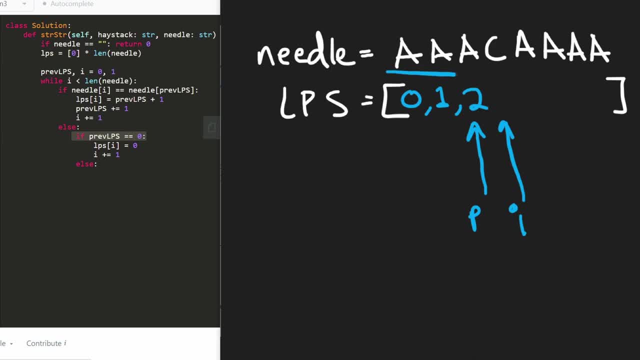 this example. so remember what this two tells us is that the first two characters matched the last two characters when we were over here. so we're trying to take a shortcut. we're trying to say, if this character matches this character, then we can put a three here, because that means these three. 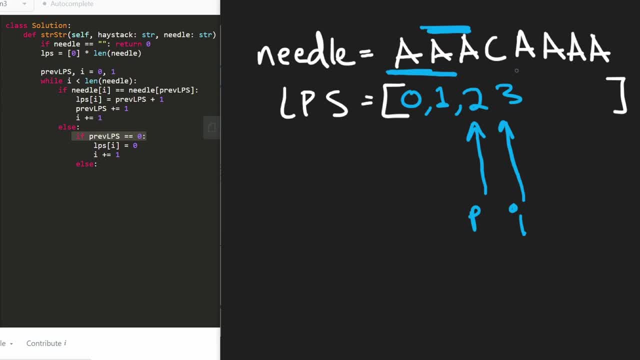 match these three, but if they don't match each other, that tells us the longest prefix suffix of this spot cannot be three. that's what we were trying to check. can it be three? right, we were using the previous work that we'd already done, but now we know it can't be three, so we're going to 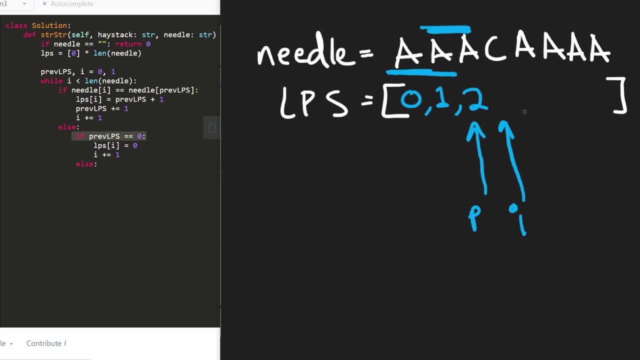 be three, but maybe it can be a two value, right, how can we check if it's a two value? well, we're still going to leave our i pointer here because we're trying to fill in this spot, but our p pointer, which was over here. now it's going to be shifted to whatever value happens to be, to the 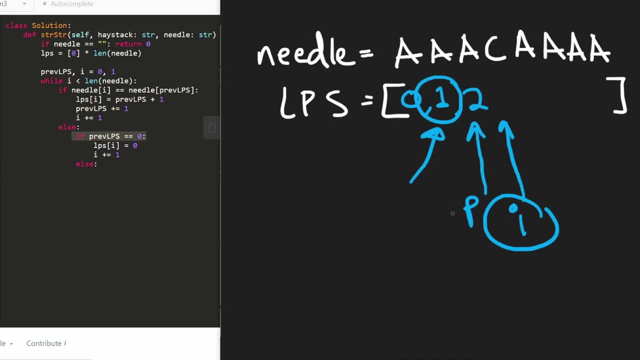 left of it, not necessarily decremented by one. right decremented by one would be just putting it over here, then putting it over here, etc. etc. but we're going to move it to whatever value is to the left of it, which, in this case, is going to be the left of it. so we're going to move it to. 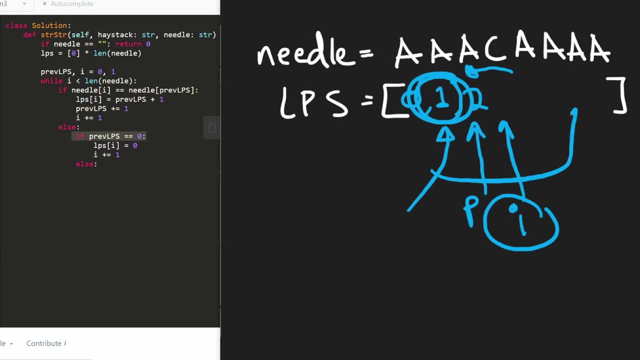 decremented by one, but it's not always going to be the case, as you will see when we finish this example. so for now, we're going to take our p pointer and actually set it to be over here now, and what that tells us in the context of this problem is we're going to be using a shortcut to 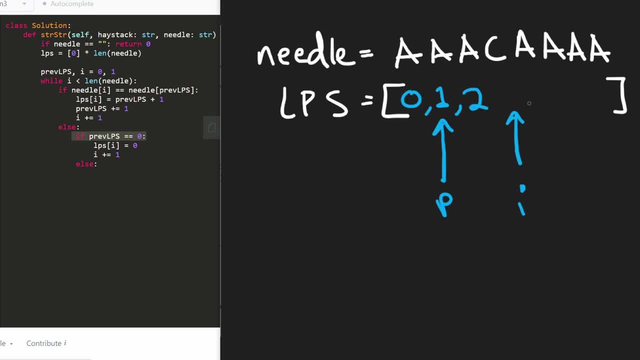 check. can we put a two value over here, because we already know that this character matched this? that's what the one tells us, right? the prefix here was one, so the one character from here matches one character from this, and we already know that this character matches this. so we're going to be. 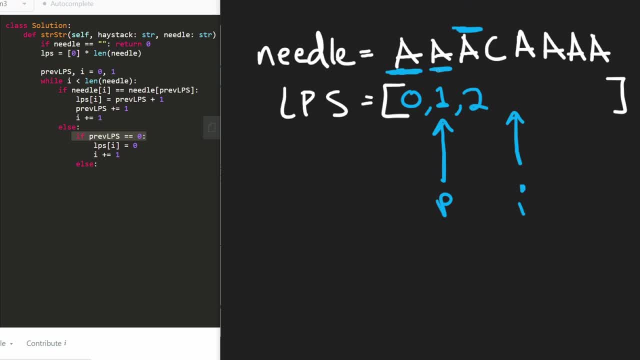 here. so now, if we know that this character matches the c character over here, then we can put a 2 value here. right, we only have to make one comparison to determine that. but again, these characters do not equal each other. the a does not equal the c, so we can't even check that now we're. 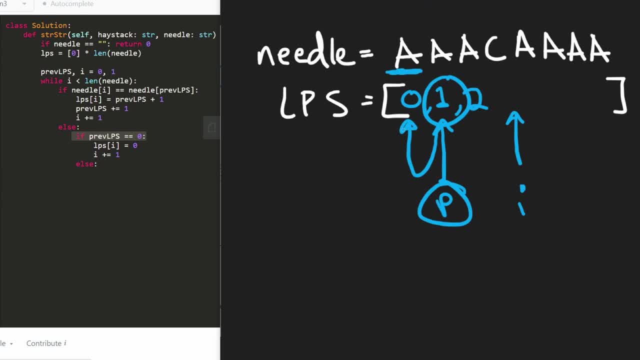 going to take our p pointer, set it to whatever value is to the left of it. right now it happens to be zero, so therefore our p pointer is going to be decremented by a1 and we're basically now to the point where our p is all the way at the beginning of the string. so i was talking through. 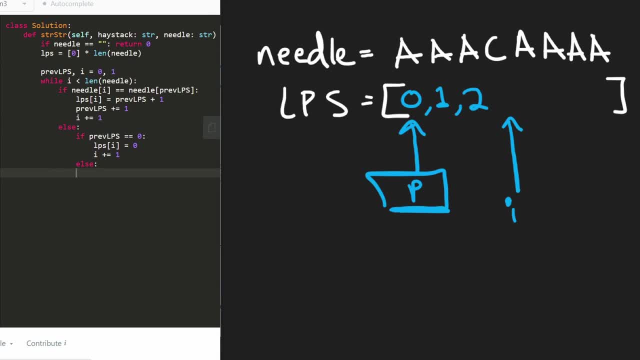 this, but i probably should have coded it up at the same time. so let's just fill in our else case to set the previous lps pointer to be equal to lps uh at the you know index of a previous lps minus one, right. this is the value our previous lps pointer is going to be set. to notice we don't. 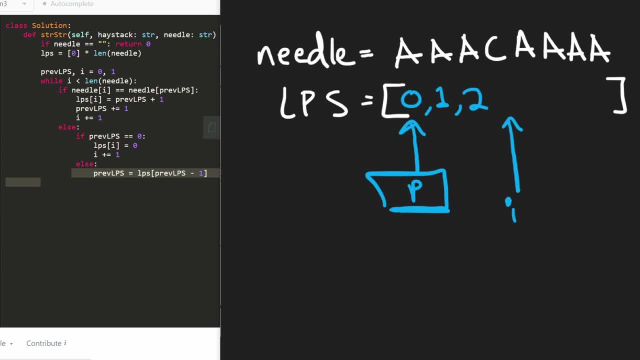 increment our. i pointer here because it doesn't really make sense in the context of this drawing and if it makes you feel any better. this actually is the entire code to set up this lps array, even though it's quite complicated. but let's just run through the rest of this example and actually 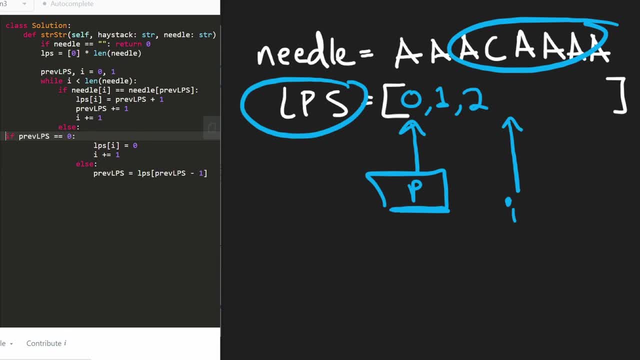 since we have an else if here, we can, uh, you know, condense this to this being an else, if and this being an else. okay, so now let's run through the rest of this drawing. so now our p pointer is here. since this is a zero, that basically tells us we're not even using any. 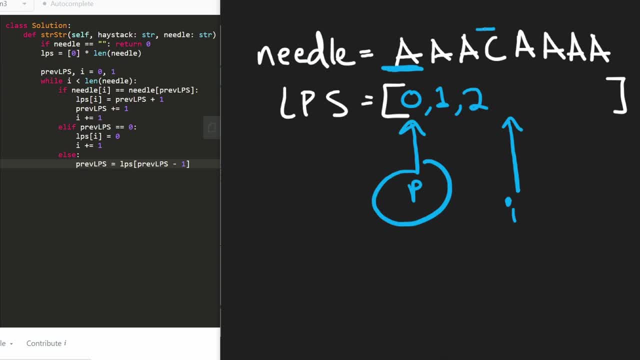 of the pre-work that we did. we're directly comparing the first character with the last character. can we at least put a one here? is there at least a prefix of length? one that's equal to the suffix of length? one that's not even true, though. the c does not equal an a. 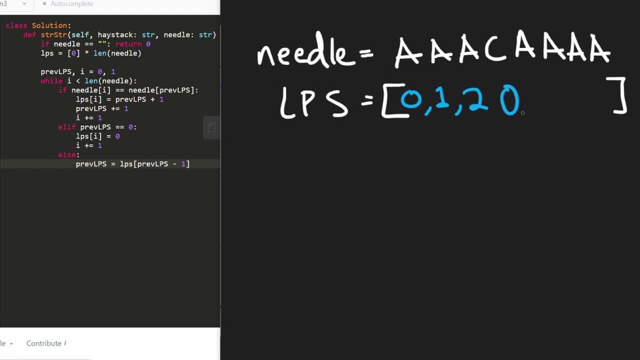 so we have to start all over. this is going to be a zero value, right, and the reason we're putting a zero value here is because now we're executing our else. if, because our previous lps is already all the way at zero, right, this is where our previous lps is. we can't decrement it any further. 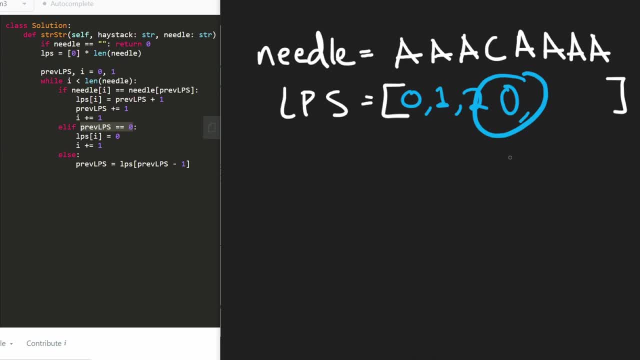 so that's why it stays here and we continue to the next position. we're going to be using our previous lps as an addition, where our- i pointer uh- will now be over here and our lps is actually still going to be. our previous lps is still going to be over here. okay, now we're going to start. 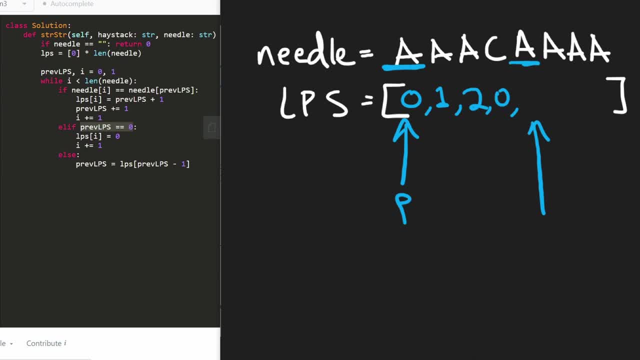 building our way back up, because this character does match this character, so we can set this to previous lps plus one. previous lps is zero, so we can set this to be 0 plus 1. that's going to be one. we're gonna uh, and, by the way, actually our previous lps is also going to be incremented by. 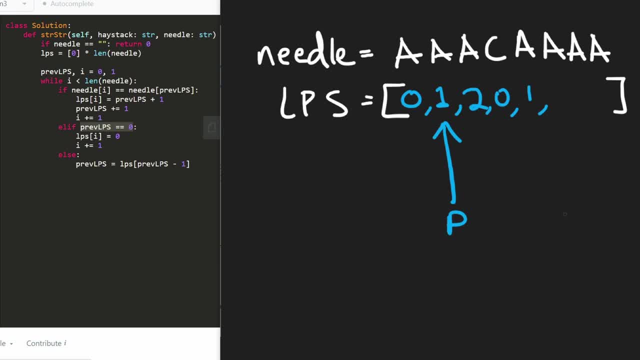 one, since we found matching characters. so this is going to go here. right, and our- i pointer- was also incremented by one. now we're at this character, and what does this mean? our, our previous lps, is at index one and the value at index one happens to be the value one. 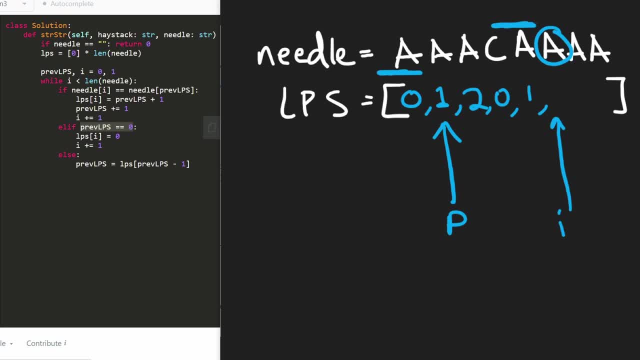 it means that the first character already matched this character. that's why we incremented this to one in the first place, right, because that's what we just checked. we checked that this is equal to this, so therefore we only have to compare this with this over here to to set this equal to two. 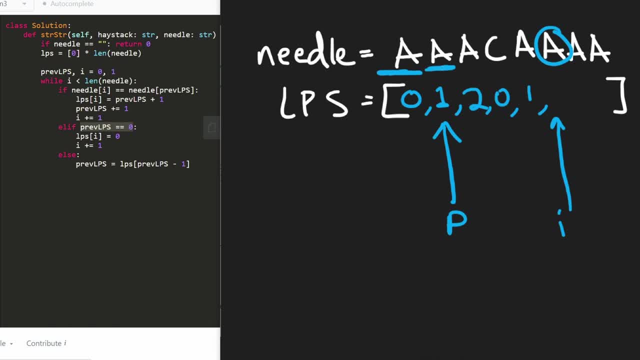 right, we're trying to shorten our work, they do happen to match. this matches this, so therefore we can set this equal to two without having to re-compare these. right? we know that the suffix of length two here is equal to the prefix of length two here. and again, we're going to look. 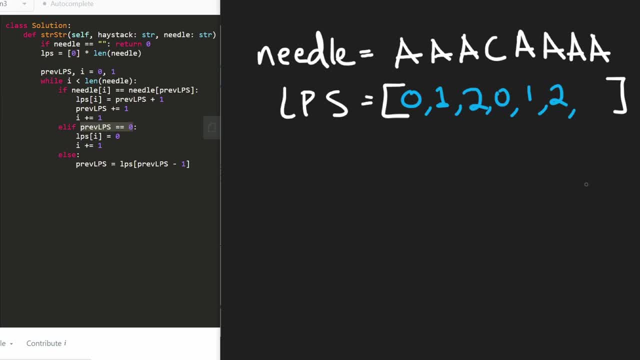 at this character and this character- and, by the way, our i pointer is going to be set to here now, our p pointer is going to be here- that means that these two match these two already. so all we have to check does this character at the p pointer? 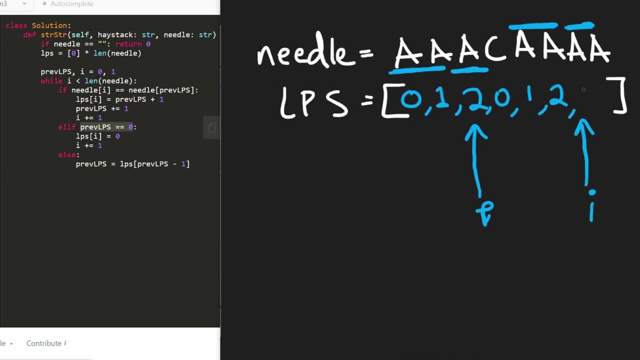 match the character at the i pointer over here. yes, they do, so we can put a three here now. this is the part where things are about to get interesting. the last index. so our i pointer was over here, right, we incremented it by one. our p pointer was here, but now we increment it by one. 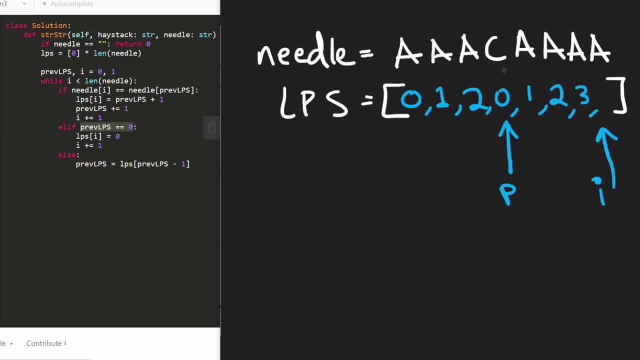 to be over here, since we found matching characters and what we're trying to do, remember, is shorten our work. we know that these characters match these three characters and we're going to that's what we determined by this, So that's why we only have to compare this character with this. 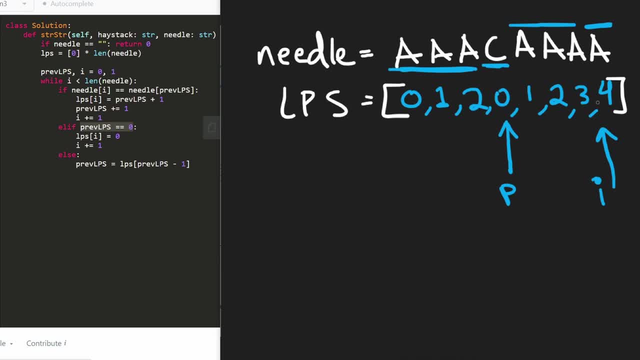 one to be able to put a four here, but they're not equal right, So that means we're going to execute our else case. does previous LPS equals zero? it does not equal zero. just because the value here is equal to zero does not mean this is equal to zero. this is equal to four, as you can. 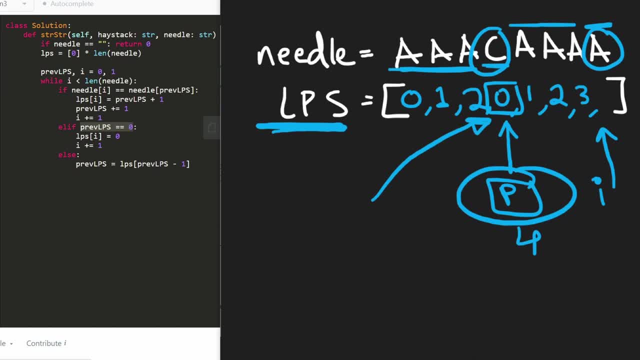 see right, it's at index equal to four. So that else, if case over here is not going to execute, we're going to execute the third case And let's see what it ends up doing. So this pointer is going to be set to the value at the index to the left of it. So it's going to be set to two. 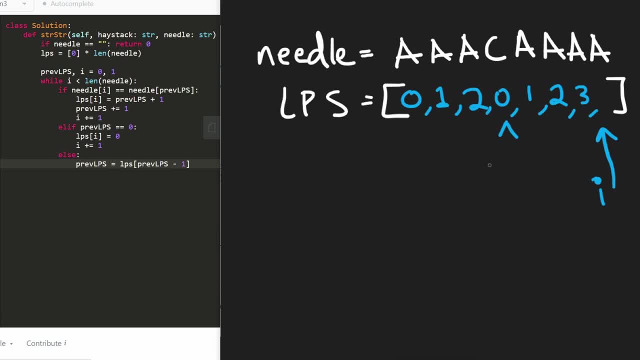 which happens to be this position itself, right? So our P pointer is now going to be shifted all the way over here. So now, what does that mean? Because now the loop is just going to execute one more time And it's going to run through these same conditionals. So now, what are we checking? 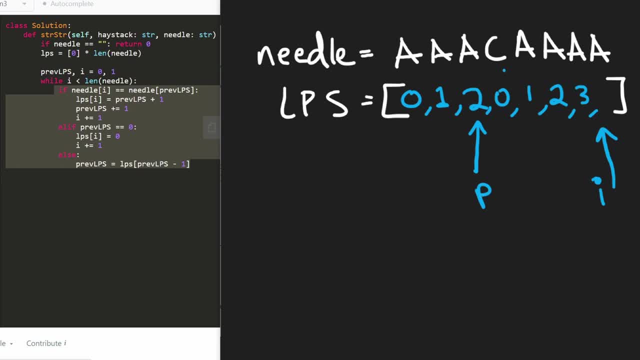 now that our P pointers here. What's different now? Well, since the value of this is equal to two, now, what that means is the first two characters match these two characters. But now we're checking: does this character match this one? if they do match which? in this case? 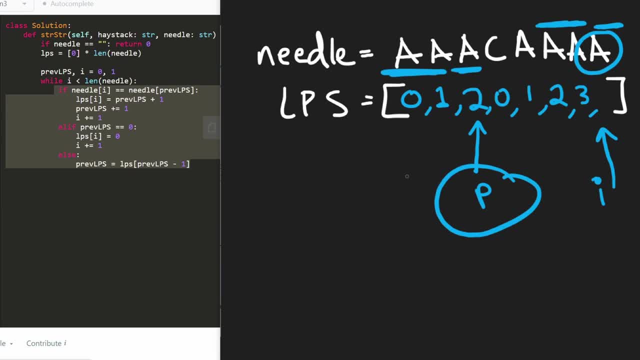 yes, they do match. we can take the value of P, which is equal to two- it's at index- to add one to it and then put that here. So we'll put a three here, right We? we already knew the first two characters match. if this character matches as well, then we set a three. 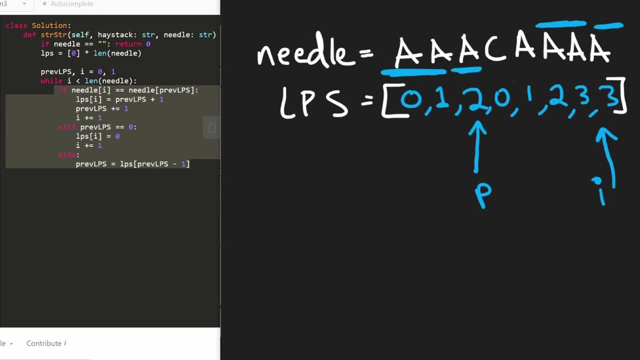 here. right, we kind of cut down the work that we had to do. So that was a lot of work just to set up this LPS, And the time complexity of setting this up is actually just going to be the length of the needle times two in the worst case. I'll show you why I won't talk too much, why that is. 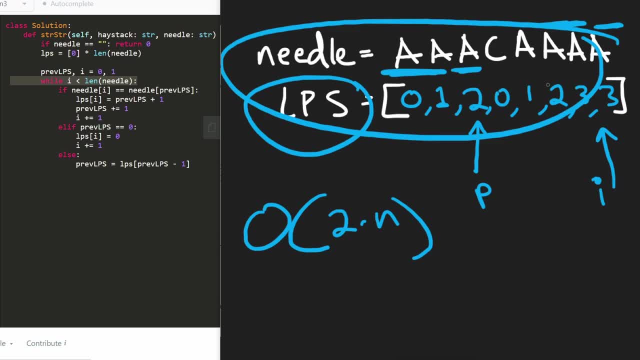 But if you kind of you know, pick any example and go through this, you'll see that we don't. you know, this is not exponential or like n squared or anything like that. yes, sometimes we have to decrement our P, But if you took the example where we just have a ton, 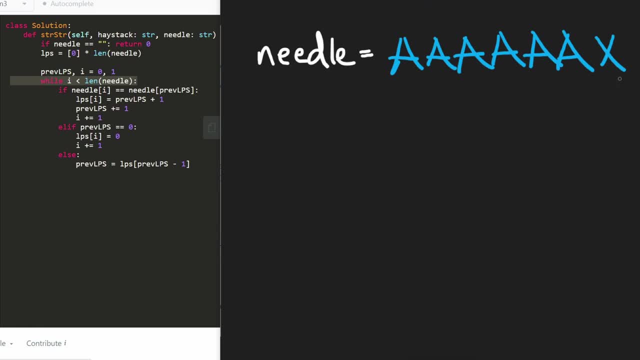 of A's and then you know, at the end of it we have like an x or something. the P pointer and I pointer will continuously be incremented by one each time, But when we finally get to the end, our P will be here, our I will be here. we're going to realize that. okay, these two are not. 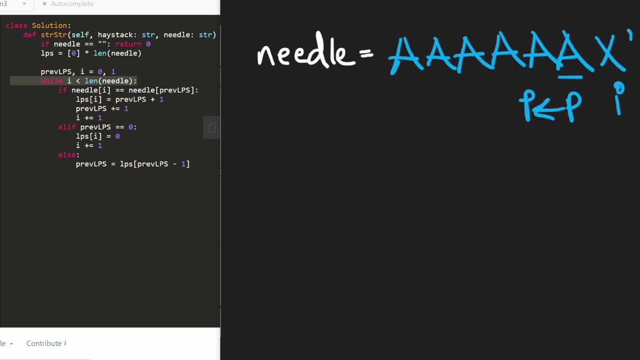 equal, we're going to decrement our P by one over here. Again, we're going to see that this is not equal to this, So we're going to keep decrementing our P continuously until we get to here. I hope that gives you an idea of what we're going to do next. So if you're interested in learning more about 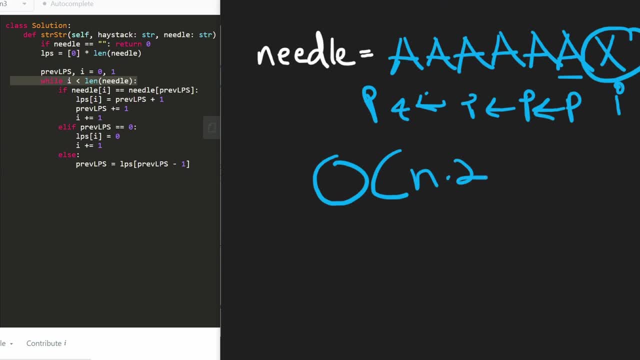 a little bit of the intuition of why this LPS is actually just two times n, not n, squared. Okay, but that was a lot of work. So now let's actually get into the KMP portion of the algorithm, now that we actually have our LPS set up, And let's actually start with the code at first. So what? 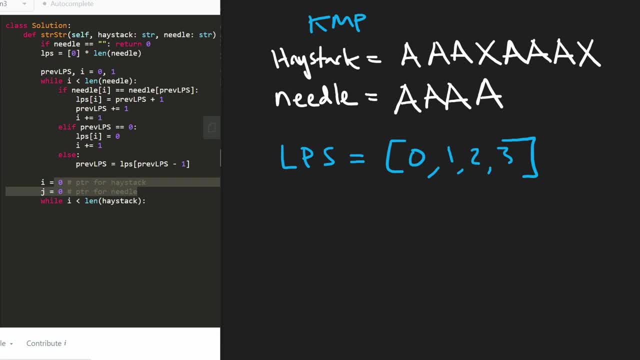 we're going to do is just initialize two pointers. I pointer is going to be for the haystack, J is going to be for the needle. they're both going to be at the beginning of each of those strings And we're going to continue this loop until we reach the end of the haystack. 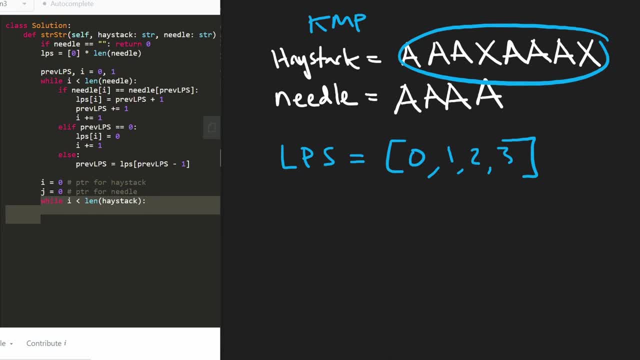 But in reality, we're also going to be having an if statement within this while loop Because, remember, what this algorithm is trying to do is, at least for this leak code problem, we're trying to find a matching substring, this needle substring, within the haystack, And, if we do find it, for 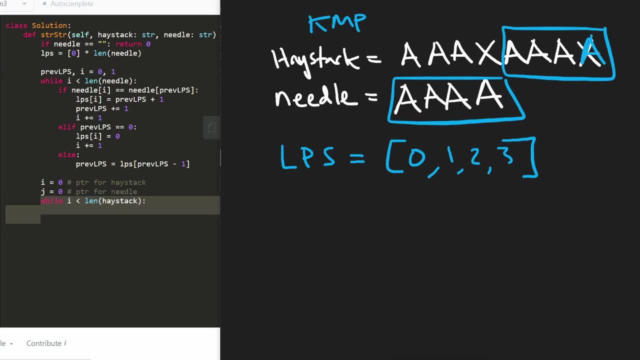 example, let's say we found it over here. if we just change this x to an a- this is the first place that we find this needle- then we're going to return the index of the starting position in the haystack where we found it. So the index of the starting position is going to be the starting. 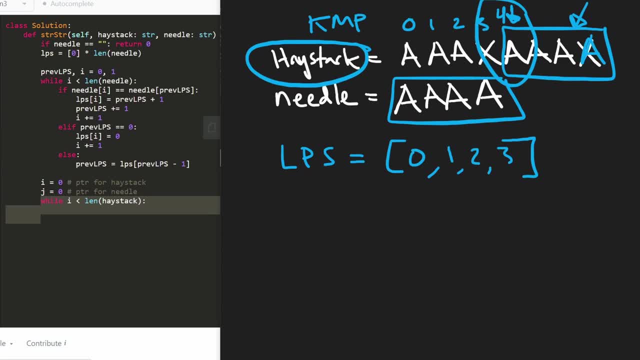 position And the index would be 01234 would be the index of this. So that's what we would end up returning. So our pointers are going to be at the beginning of both of the strings we're going to check. are they equal? that's the first thing we're going to check, right, because we want to find all 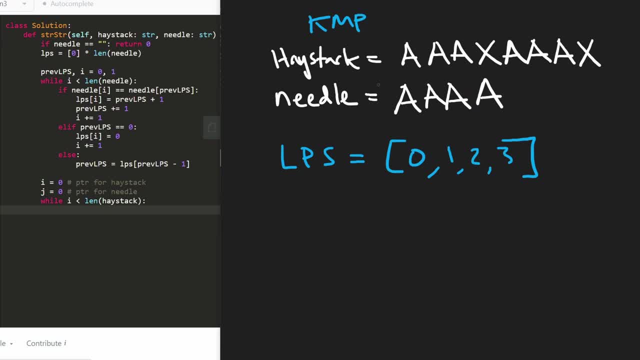 equal characters until maybe we find a mismatching character. So let's add that as a condition. So if haystack at index i is equal to the needle at index j, then all we want to do is increment both of the pointers, So i plus one, j plus one. And we probably also know that there's 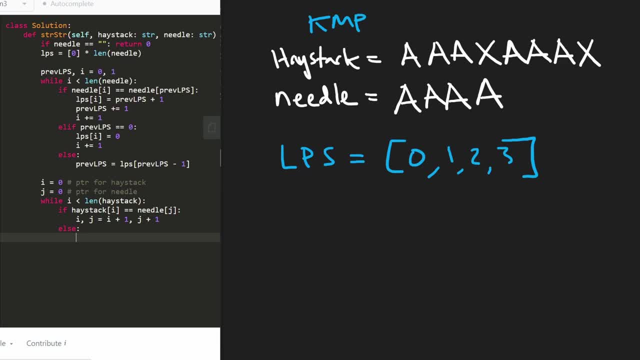 going to be an else case that's coming up if they do not match each other. So now our j pointers. here are i pointers. here again they're equal. So increment again. now they're here, again, they're equal. Now we finally get to the else case. they are not equal, right? So before we even get into 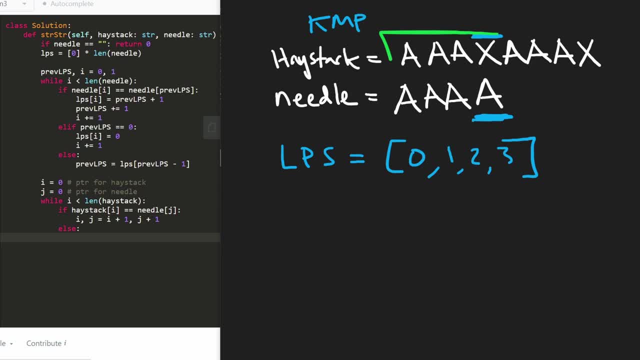 the code. let's just understand what we're now going to be doing. We were trying to check: is this equal to the needle? Now we know that the last character didn't match, So in our brute force solution, what we would want to do is now compare these four characters with the needle And 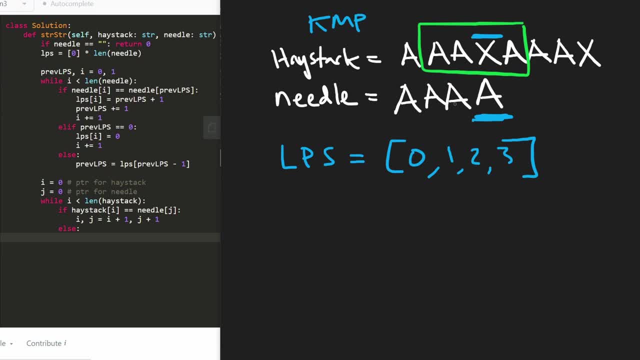 that's actually what we're going to do in the KMP algorithm as well, But in the brute force we would end up resetting our j pointer to the beginning and have our i pointer also be at the beginning. But we're not going to do that in this case, Because what we just determined right now is that 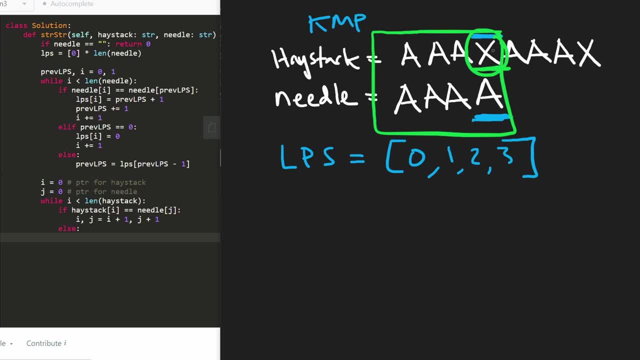 this was the position that we found a mismatch at right. this fourth position, So everything before that position was matching right. this was equal to this, And now what we're going to end up doing is shifting by one. looking at the next four characters: Take a look at this box because it's very important. the next: 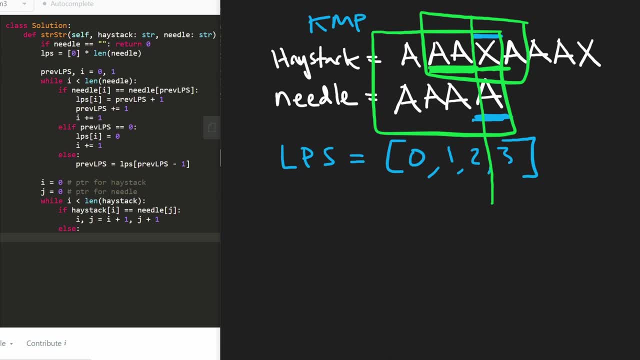 four characters means that these two characters are going to be the are consistent, right? These are the same two characters we were looking at before these over here. So this was the last matching index, Right? So now we're going to look at the position of our LPS at the last matching. 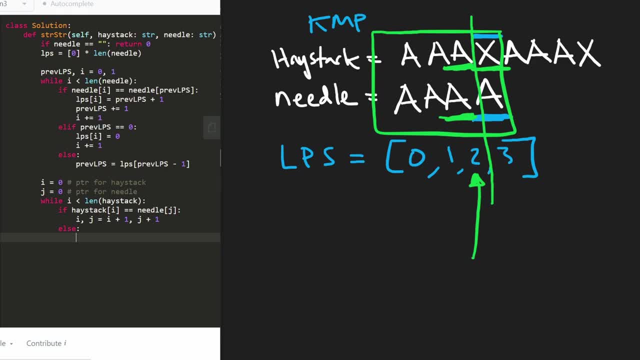 index, which is going to be J minus one. So let me just write that in the code LPS of J minus one, That's going to be important for us And in this case it's a two. What does that tell us? That tells us. 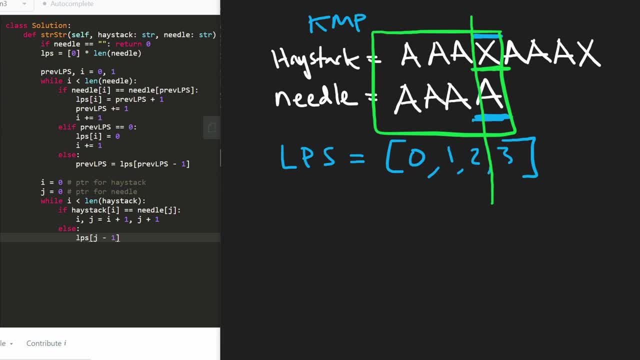 that of these two strings, the longest prefix suffix is length two, meaning these two first characters match these two last characters, even though the whole string actually matches each other. We're only going with two for now, and you're about to finally see why, Because now that 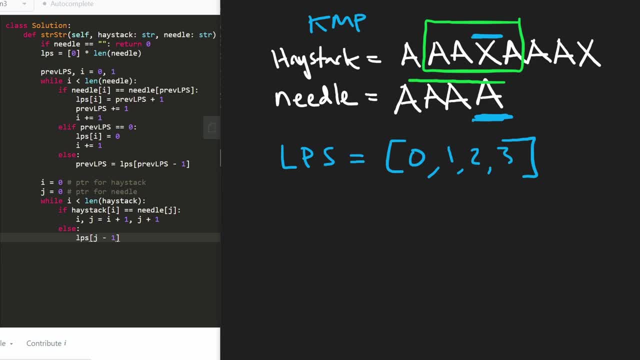 we're looking at these next four characters and still looking at this same needle. we're not going to start at index zero. We're not going to start at index one in the needle. We're actually going to start at index two in the needle because we already know that these first two characters 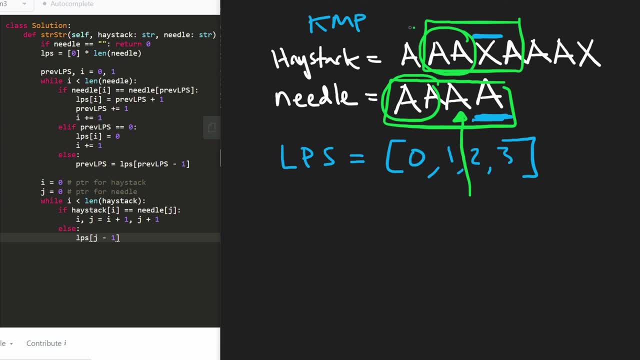 already match these two characters. Yes, we had to chop one of these off because we did have to shift our words. We had to shift our words, We had to shift our words, We had to shift our words window to be at the next position. but we still know that the two characters do match, right, that's. 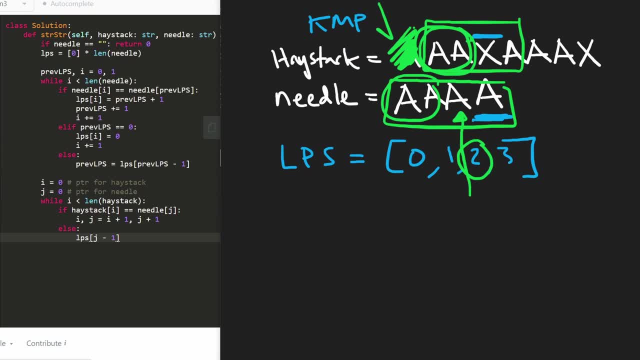 why we couldn't have done the entire three characters, because we have to get rid of one of them anyway. so, yeah, so that's the repeated work that we're cutting down on. you finally kind of get the big idea that we were going for. but, that being said, originally our j pointer was over here. 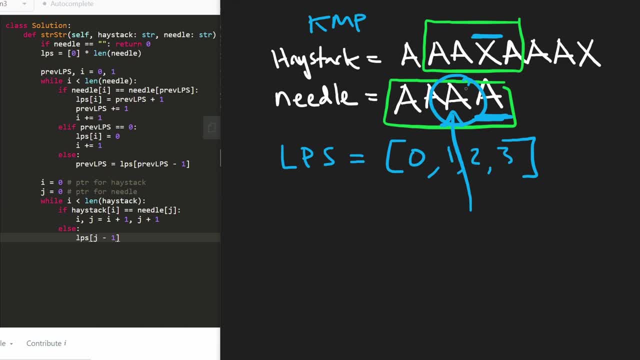 uh, but now it has to be over here. yes, it had to be: uh, decremented by one. uh, but not literally decremented by one, because now in the code you're about to see, uh, it's going to get a little bit complicated before it gets simpler, but what we're going to say is: if j was equal to zero. 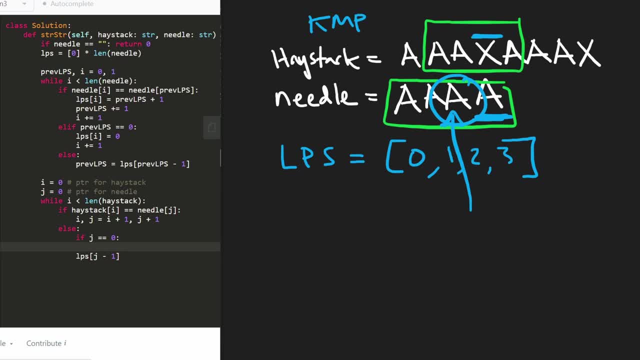 meaning we were at the beginning of the needle. we're going to handle things a little bit differently, uh, compared to if we were, uh, in the middle of the needle, and that's going to make sense in just a moment. but for our else condition, where we are not at the beginning of the needle, instead of setting 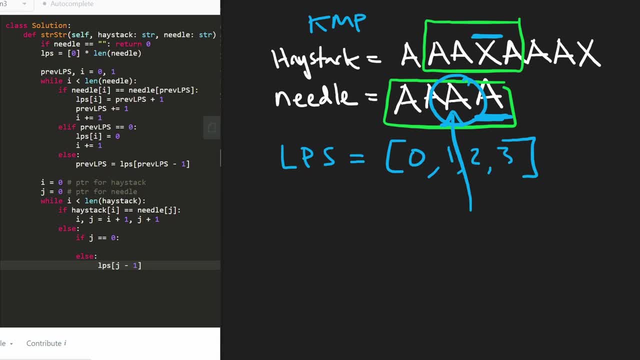 our j pointer all the way back at the beginning right. instead of setting it equal to zero, we're now actually going to set it to b lps of j minus one right, whatever however many characters were matching. in this case we had an lps longest prefix suffix of length two, so we were able to set our j to be at index two because we 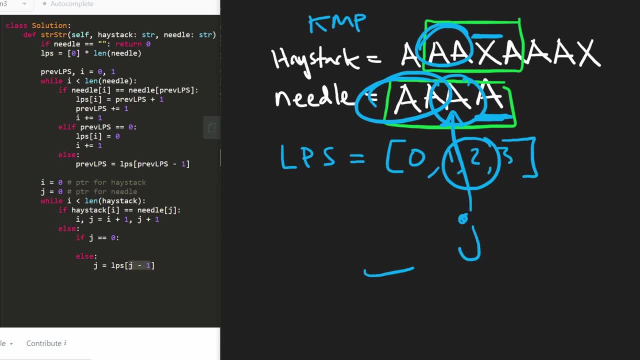 already knew the first two characters matched the last two characters of the haystack matching portion, even though our j pointer is over here. now, right, we don't have to go through these first two characters. our i pointer is still over here, right? we were looking to match this x character and we're 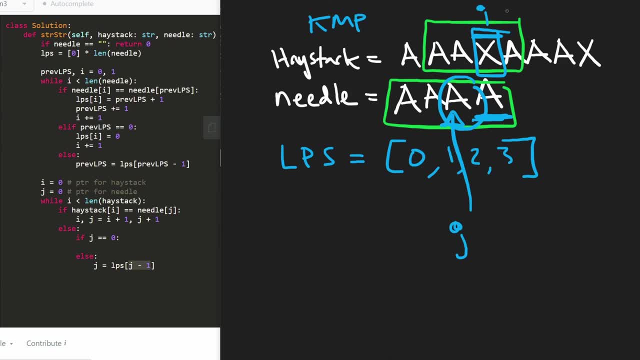 still over here, right, so we're still over here. right, so we're still over here, right? so we're still looking to do that. we can't just skip this x quite yet. okay, so now we're going to continue to the next iteration of the loop. we're going to check: is j equal to i? again, they're not equal. 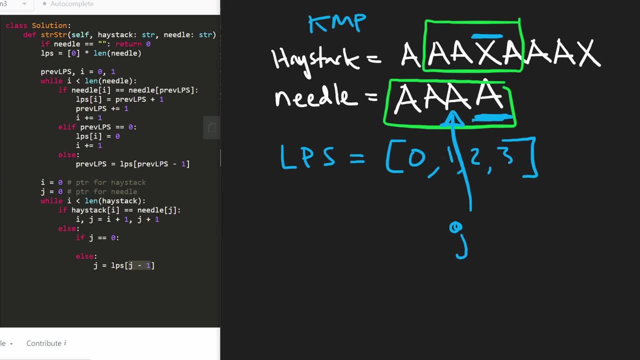 to each other. so again we're going to run our else case. and again j is not equal to zero right now it's equal to two in the second position. so we're going to again set it equal to lps of j minus one. lps of j minus one means at index one, and just for the context of this problem. 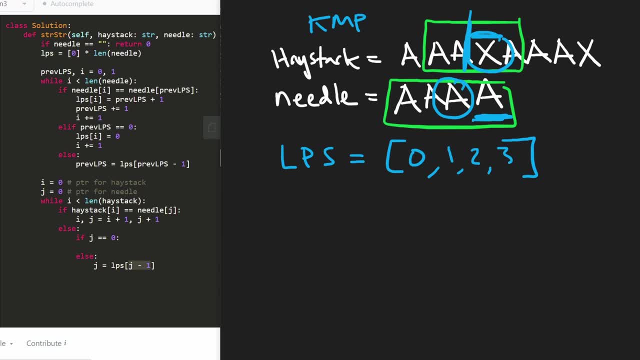 you know, this character is being compared to this character, meaning that these two characters, as we know, already match these two characters over here. right, what's the longest prefix suffix with this string. it's one right. this matches itself. so now that our j pointer is actually going to be pointing, 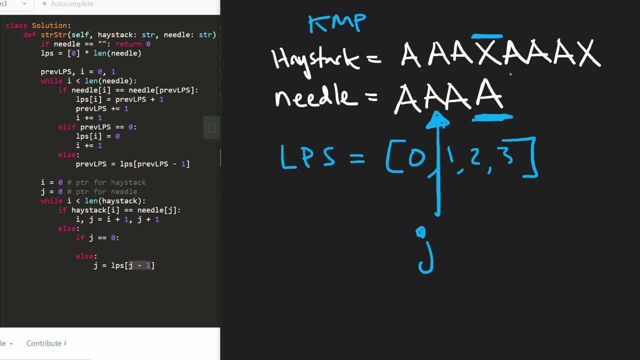 over here at this second character. what that still tells us is, though, even though, yes, we shifted our window by one and now we're comparing this with the x character, we still know that the first character of this is equal to the first character of this character, of this character, of this character. 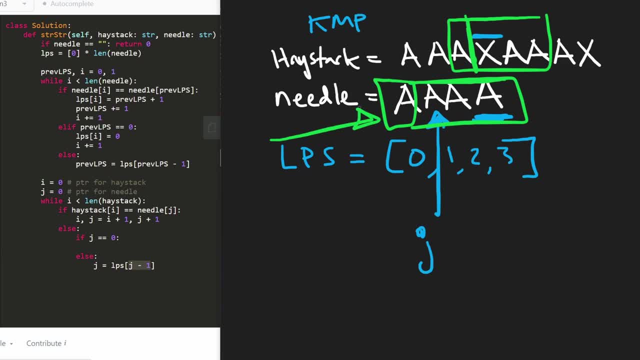 over here so we don't have to re-look at this first character. that's what the lps saved us, but, as you're about to see, it can't save us forever, because now we're going to run the condition again, we're going to run the loop again. does this a equal? this x character? remember our i pointer? 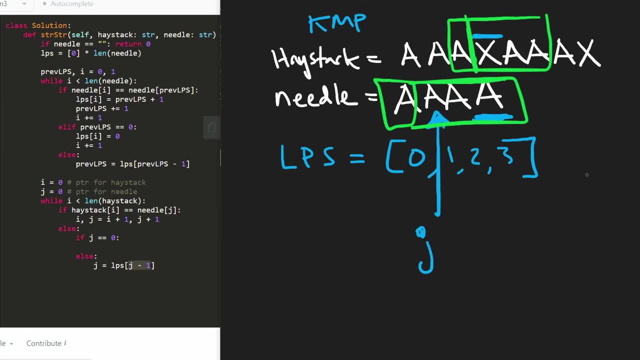 is still going to be pointing at the x. they're not equal. again, now we're asking: what's the longest prefix suffix between uh, these two characters which do match each other, right? this string? it's zero. right, basically, our j minus one, it's zero. so now, as we shift our window one more time, now our window is shifted all the way over. 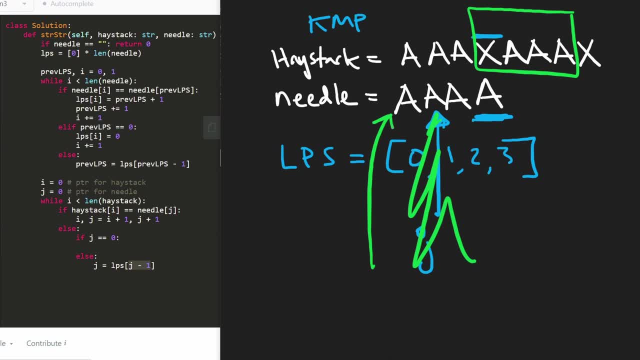 here. our j pointer is actually going to be over here at this first character. so now, at this point, you might be wondering: is this about to go forever? like, how are we going to fix this? our j is over here. it's still not equal to the x, so what exactly can we do? uh, well, that's where our if statement. 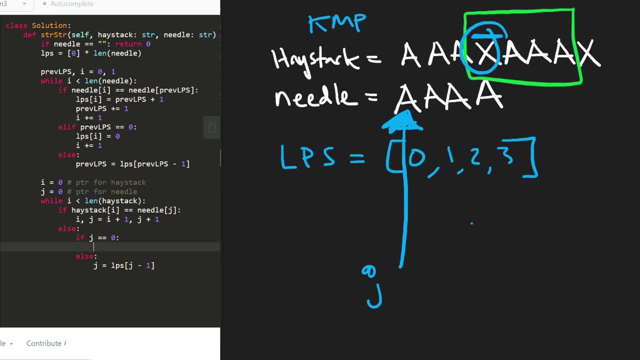 over here comes in, we have an. if j is equal to zero, right? what can we do now to stop this from running forever? well, logically, in this drawing, what we would want to do is still shift our window by one. right now, we want to look at these next four characters. so this is actually 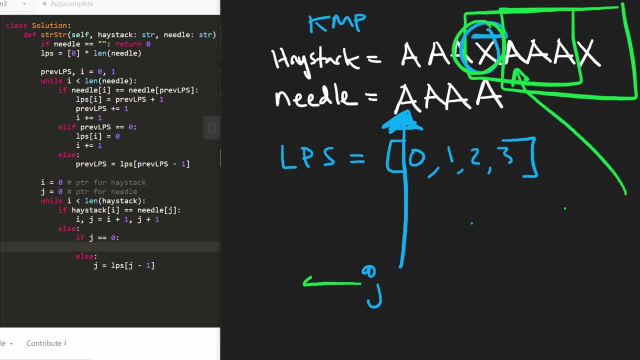 not even available anymore, so clearly can, since we can't shift our j anymore to the left. what we're going to do now is just increment our i pointer, and now you can finally breathe a tiny sigh of relief, because that's the entire algorithm, except for one last thing, and i'm actually going 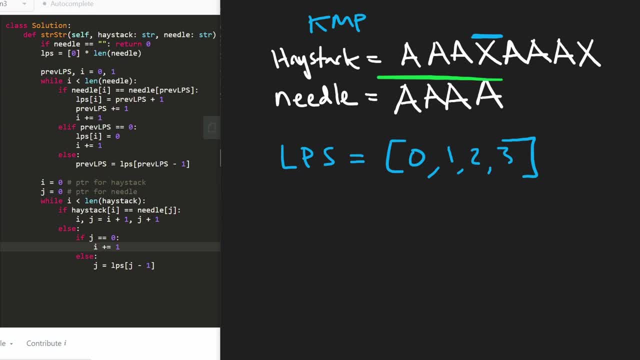 to slightly change this example because, as you can tell, this is never going to match anywhere in this string. so let's actually change this x character to be equal to an a character. so right now, our i pointer is over here, j is over here. these characters do match each other, so we simply increment both of the pointers by one, as you. 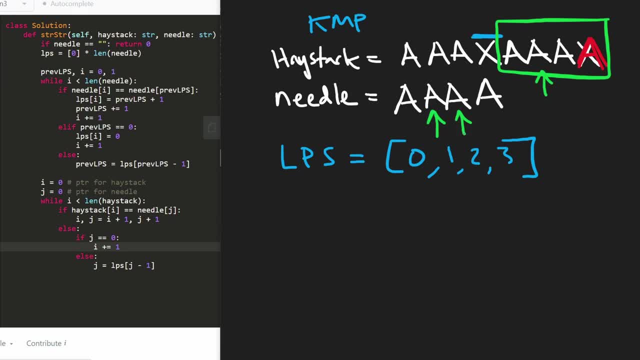 can see on the left side with our code: again they match each other. so we increment them by one. to the next character: again they match each other. so we increment them by one. and the last characters also match each other. so again, Then we increment them by one. 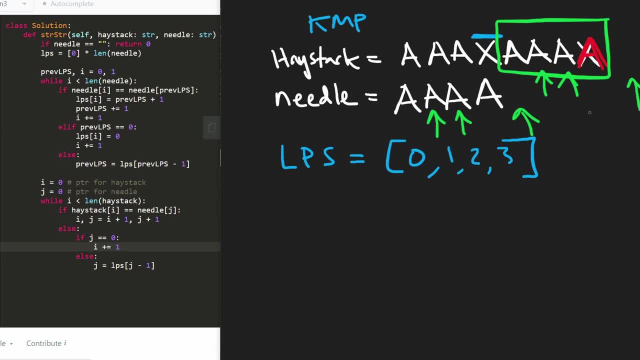 So right now, both pointers are actually out of bounds. but let's change the example a little bit more. Let's actually add a last character in the haystack. But what we found is that we reached the end of the needle, even though we didn't necessarily. 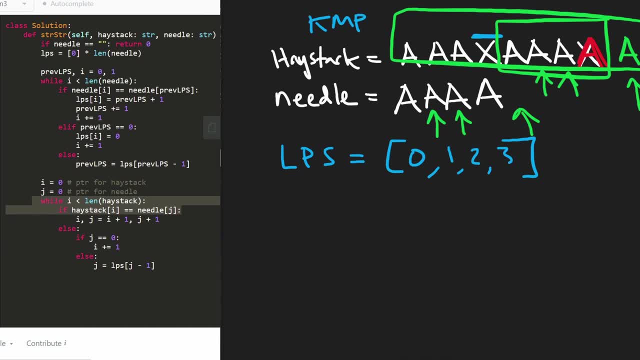 reach the end of the haystack. That means this, you know, while loop is going to continue to execute, but we don't want it to execute As soon as we find a match. we want to be done. We know we found a match because we reached the end of the needle, because J is now equal. 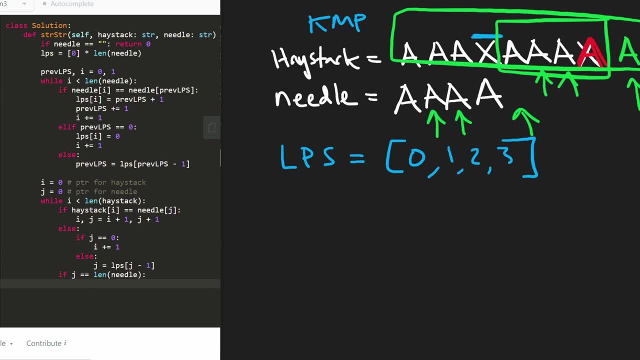 to the length of the needle. It's out of bounds. Therefore, we found a result. Therefore, we want to return the first index that we found that result. Since this is where we found the first matching substring, we want to return the first index. 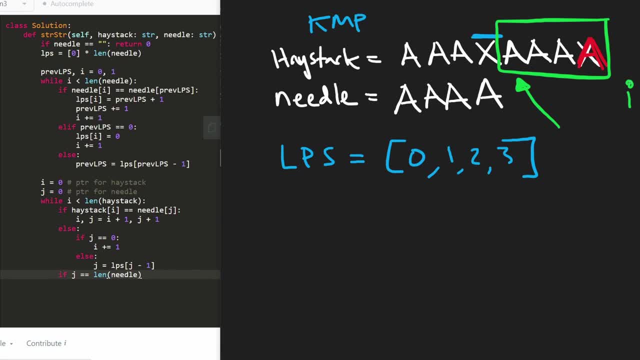 of that matching substring. Basically, we're going to take our I pointer, which is over here now minus the length of the needle, which is going to bring us bring the needle from over here to be shifted all the way to The beginning of that substring. 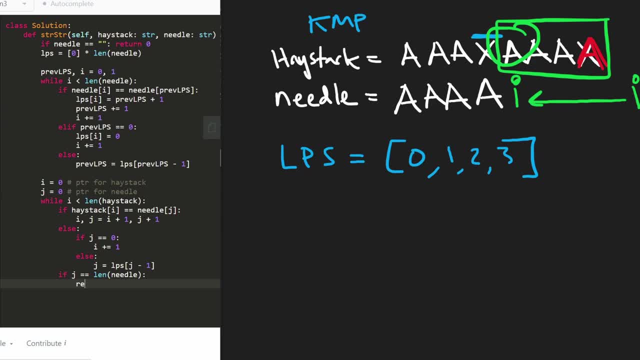 So let's do exactly that in the code: If we found a match, we can return I minus length of the needle. So that's what we're going to do, And remember: in the problem description they say that if we don't find a match, we 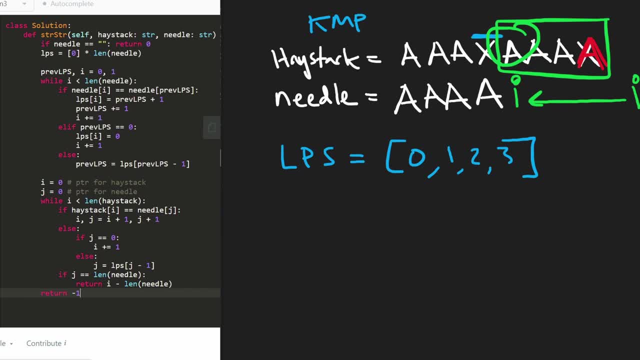 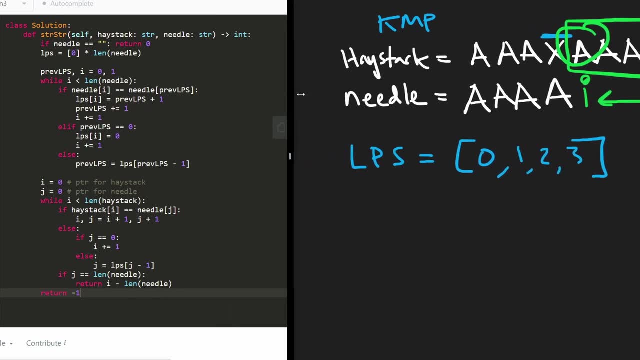 just want to return negative one, So let's do exactly that. Oh my God, that was probably the longest problem, the longest video I've ever created, But I really hope that it was helpful. Let's run the code to make sure that it actually works. 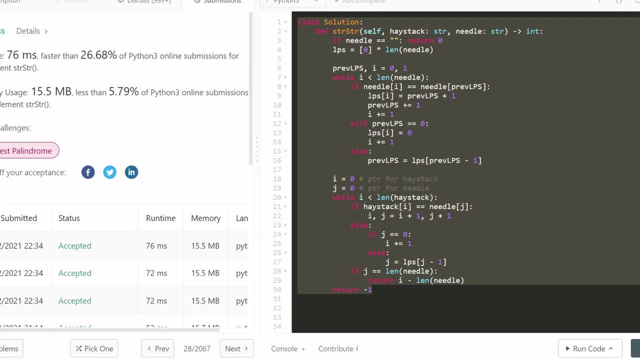 Let's run submit. Okay, Let's see if it worked And, as you can see on the left side, it's relatively efficient. Thank God it works, because I would have been pissed if it didn't after recording this for so long, So I really hope that this was helpful. 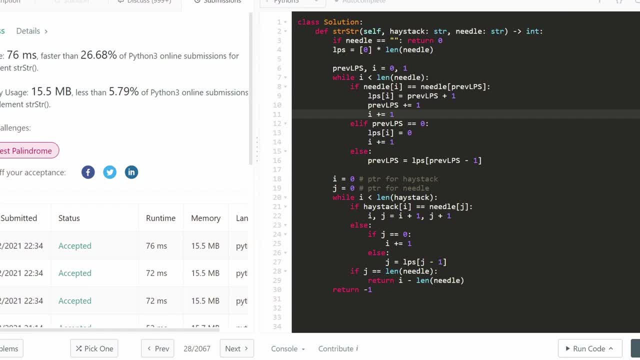 Let me know if you reached the end of the video And if it was helpful. please like and subscribe. It really took me forever to create this video, but I think it was overall worth it. I know a lot of people requested it and hopefully I'll see you pretty soon. Thanks for watching. 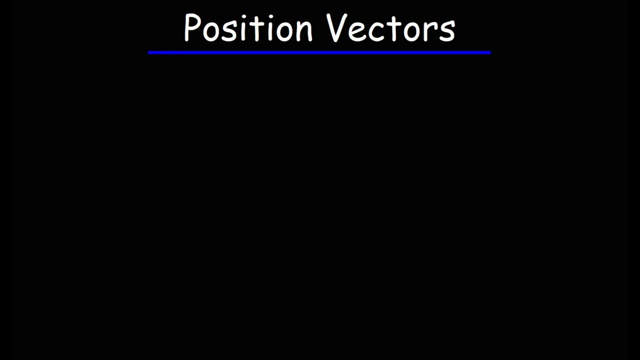 In this video we're going to talk about position vectors and how to use them to calculate a displacement vector. So what are position vectors? To answer that question, let's draw a picture. So here we have a graph. that's the x-axis, this is the y-axis.